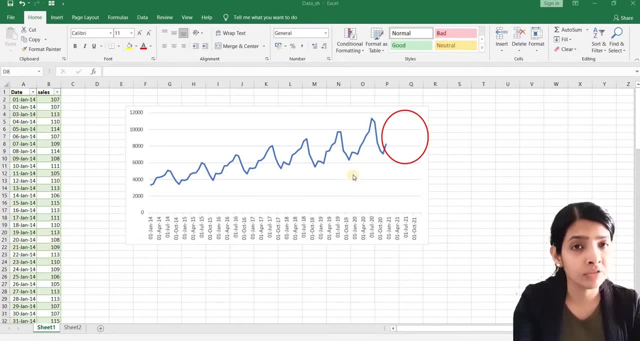 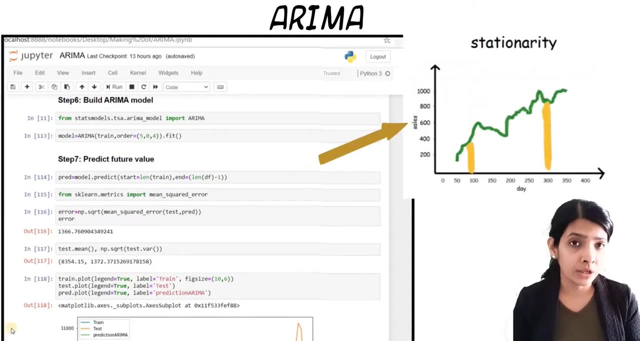 And, based on that, we would predict the sales of its next 6-7 months. We would use Python to build the model and we would understand the theory while coding. Before we start with the modeling, I would suggest you to download the notes. 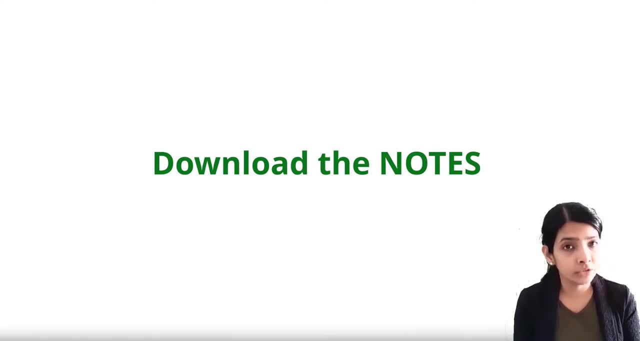 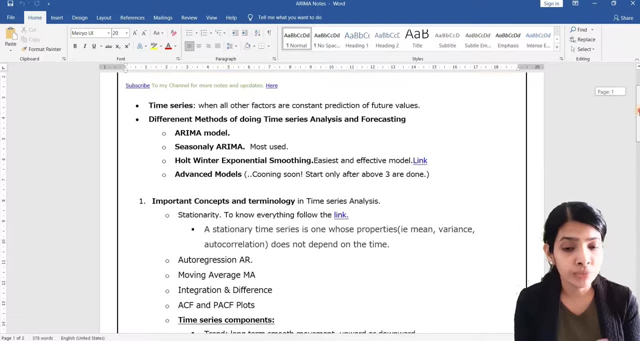 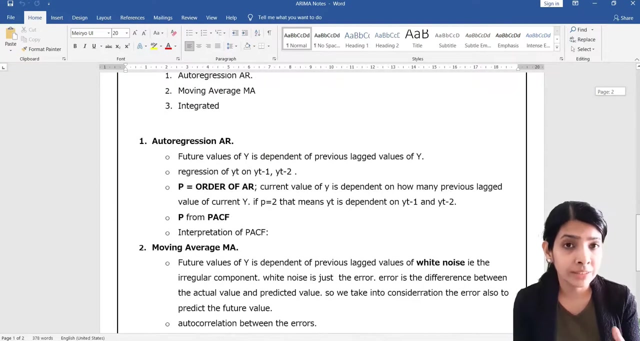 The link is given below in the description box And during this video or any other video related to time series analysis. If you find some information that is new or interesting for you, you can add that part into this note, or you can also take screenshots if you find visual descriptions that are useful, so that you don't have to search the internet every time you are stuck somewhere and you have your own notes handy. 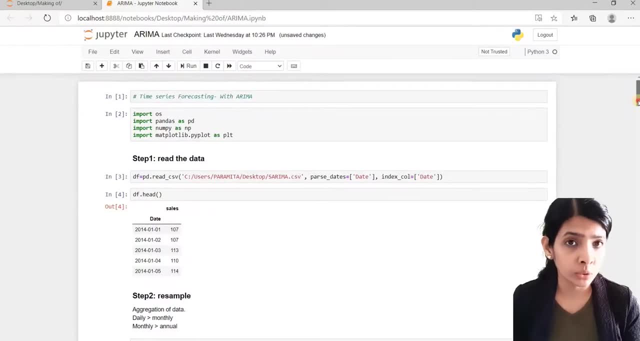 We will start building our first ARIMA model and as we move slowly, with each step, I will explain the theory that goes behind it. So we will start. So let's have an overview of what we are going to call ARIMA, What we will cover today in this lecture. 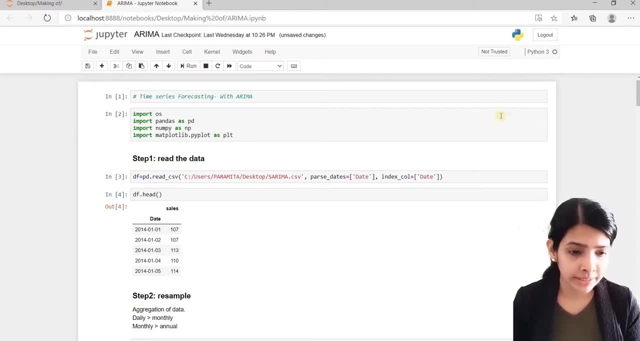 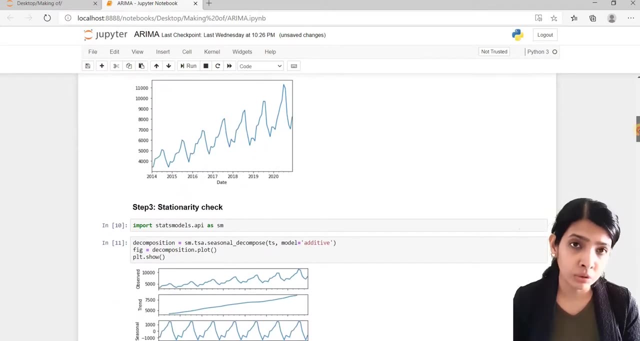 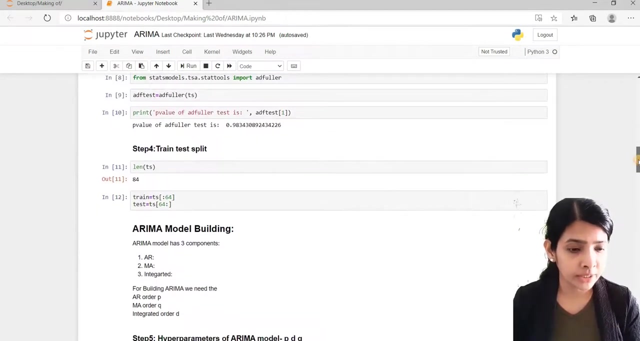 So first we would. the step one is how we read the data and step two is resampling. in step three we will do a stationary check and we will know how we do that and why it is necessary for time series analysis. Step four: we will do a trained tests split of the data and from step five we are actually moving into building the ARIMA model. 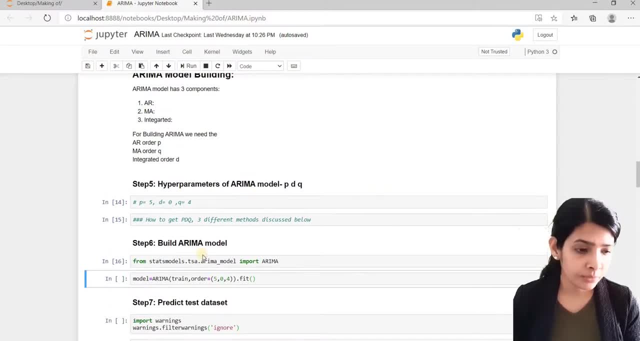 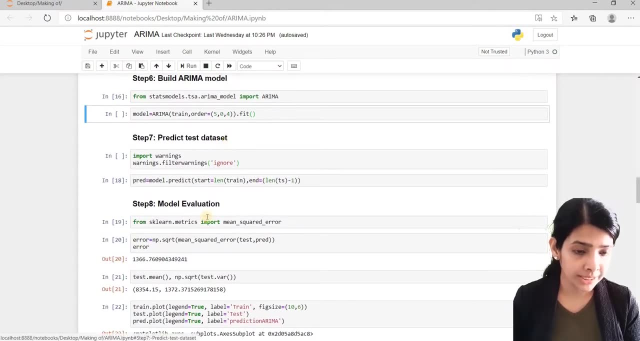 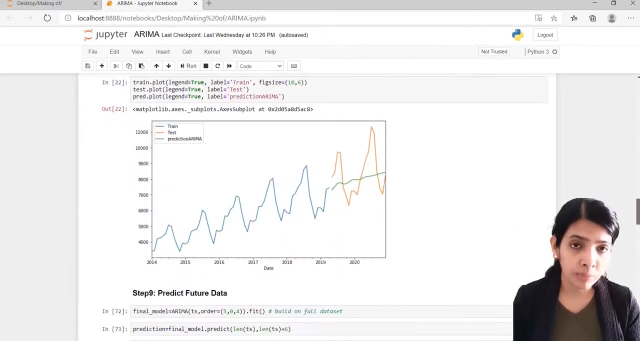 Well, we first have to decide what are the hyper parameters model. then we will build our arima model. we would predict the test data, we predict the future, future sales and in step eight we would do a model evaluation of how good our model is. we'll plot. 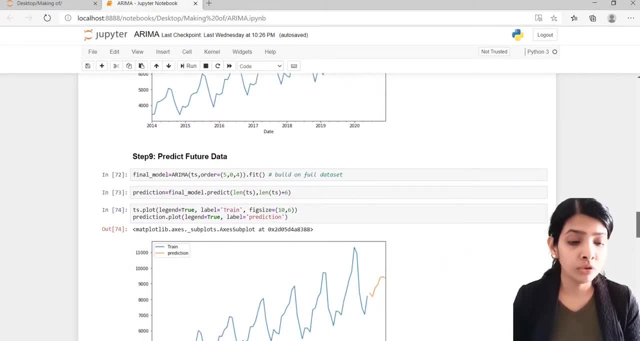 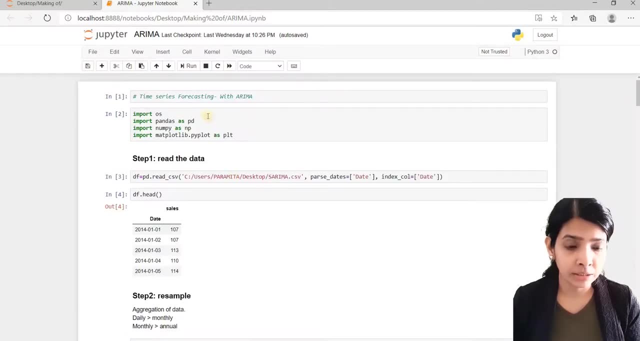 that and in step nine we would predict the future sales value, the unseen future. we'll start with importing some basic libraries that is required, like numpy, pandas and matplotlib for visualization, and whenever i need a library, i will import it right above that so that you can understand which library is used for what purpose. 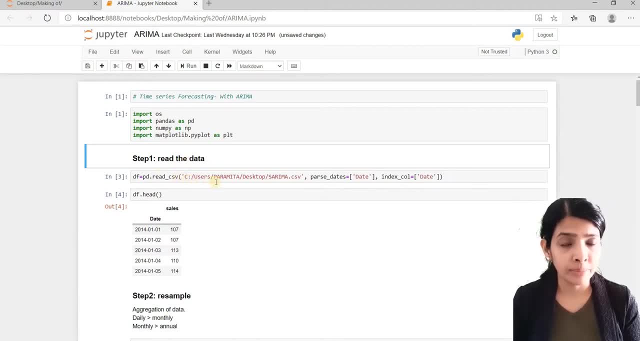 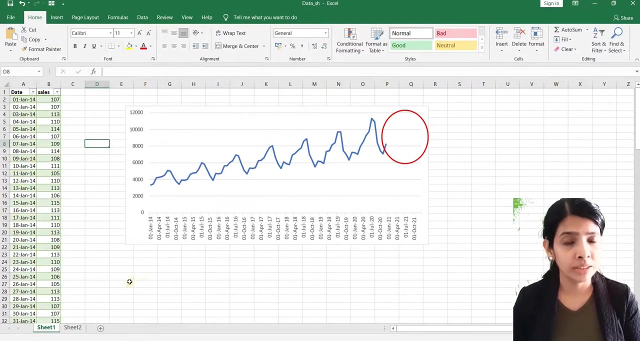 step one is read the data, and this is a very important step in time series analysis, because there are two things that we have to keep in mind. number one, that the time series model- whenever we are building a time series model, the time series data should be recorded on a fixed time intervals, like monthly, daily, it. it. 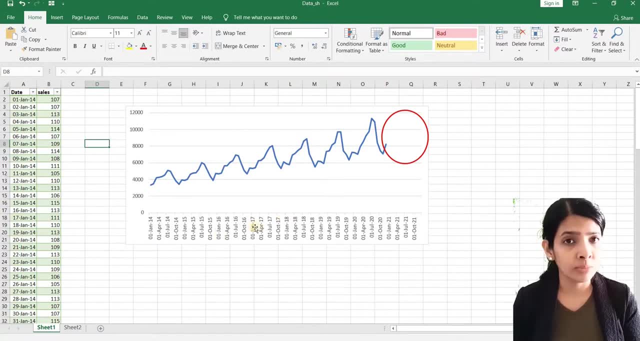 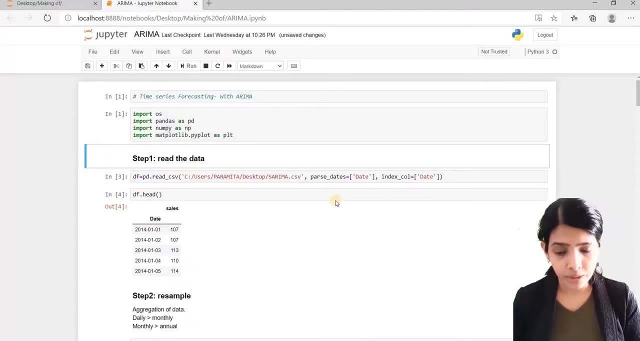 has to be regular. we cannot have the sales for two, three months and then we don't have the sales for next two, three months, so it's a irregular data. so that will not work for our time series model. okay, so in when we read the data, there are two things that's important. 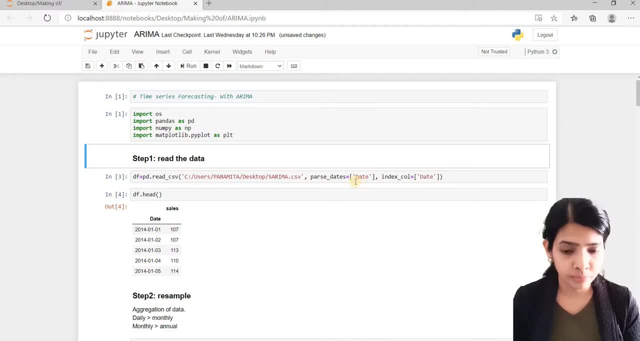 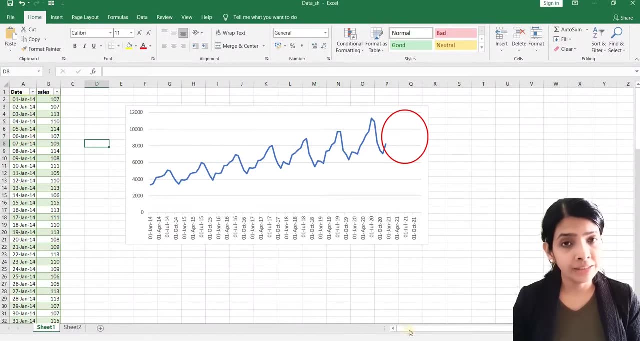 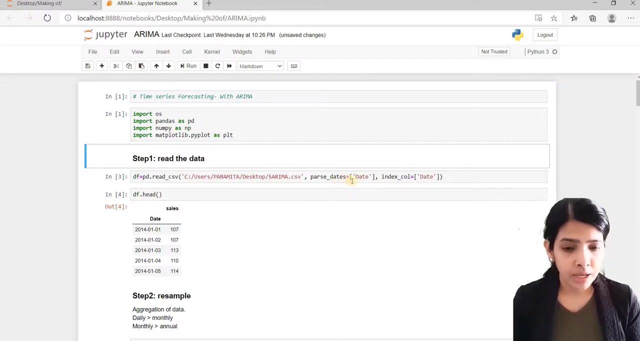 that we have to parse the column that has the dates in it. so if we parse the column, that means the python will read the dates as date format, that is, as date time object. but if we don't parse it, if we read it as plain text and for time series analysis, it is mandatory to have the dates in. 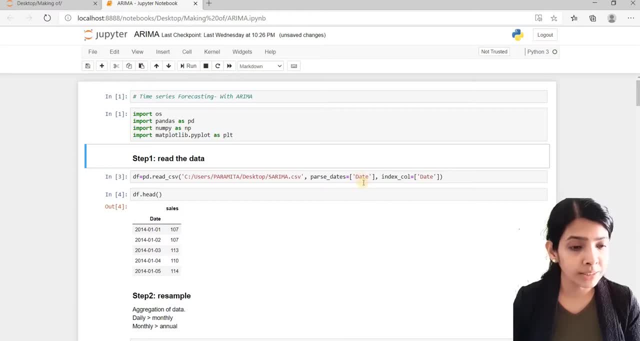 dates format only. so we would parse the data and within parse date will pass the name of the column that has the dates in it. and step number two is we would make that column that has date as the index of the data frame. so we have set the date column as index. 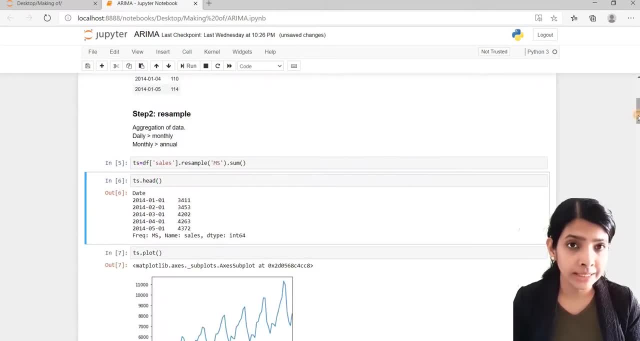 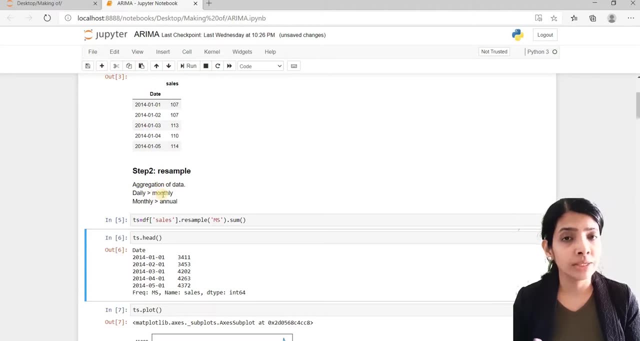 let's look at the data so we can see that we have daily sales, because sales is recorded in a daily basis. but for our analysis we need to convert the daily sales to monthly sales. this is done by using resample function. that is the step two, because in every time series analysis we have to do some level of aggregation of the data, like from. 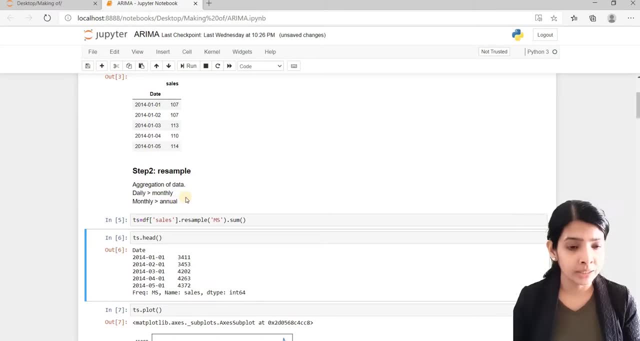 daily to monthly, like in this case, or monthly to annual data. so we have to basically group the data based on the business requirement. like here: we have daily sales that we have to group to monthly sales because sales is recorded in a daily basis, but sales reports or any analysis based on sales 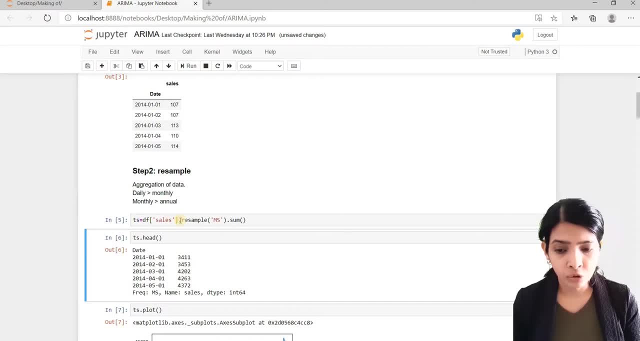 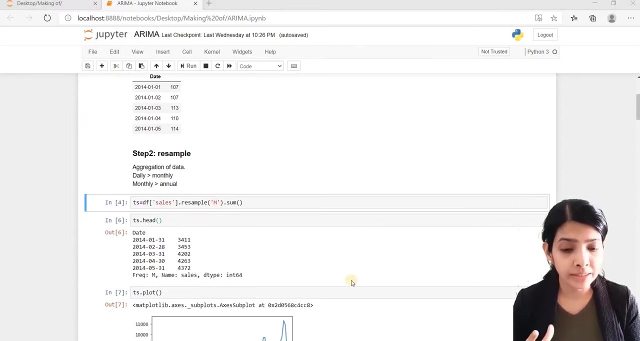 we take the monthly sales values, not the daily sales value. so we have to group the daily sales to monthly sales and we would do that by using dot resample function. dot resample is a very important step in for time series analysis. so now for annual and's respectively annual. 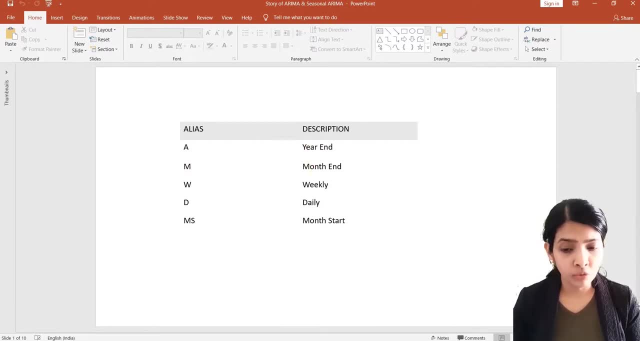 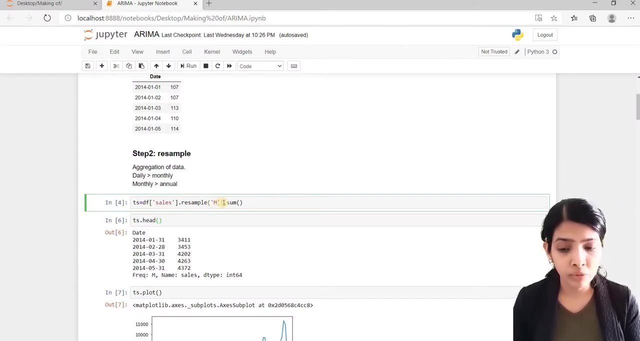 we are going to take the monthly clouds as per漂亮. here we would use the month total everyday basis chart to create the monthly sales. so from monthly sales we have to map out both of these in R2. so we need later to можешь to add on month to daily, fromk to monthly to annual. and the first step is for time series analysis. 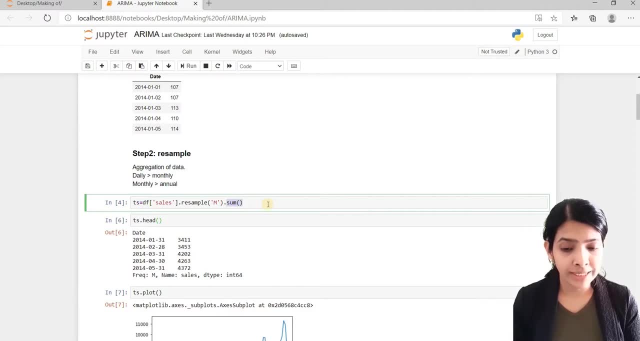 takes two argument. one is the rule. in the rule we have to mention how we want to aggregate the data. A means that we want to have annual totals, M stands for monthly, so we would resample the daily data to monthly total data. And the second argument that is needed: we can pass it as dot sum or dot mean. 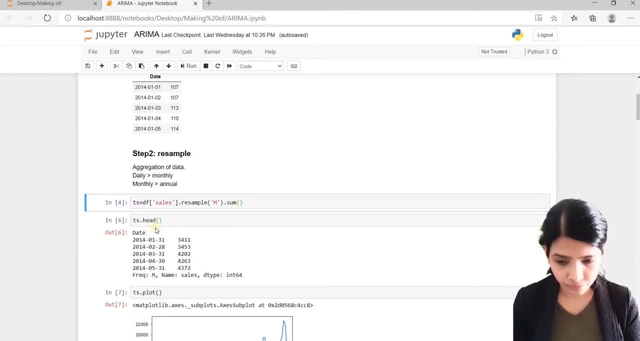 Here we would do dot sum because we need the total sales. Now let's look at the data frame. But the date here is showing month ends. But we can change it to month beginnings by mentioning the rule equal to MS And that looks better. 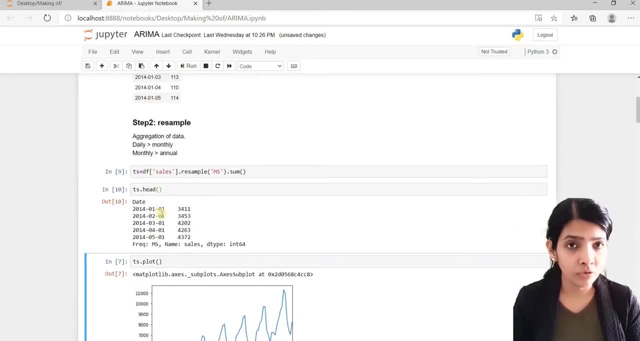 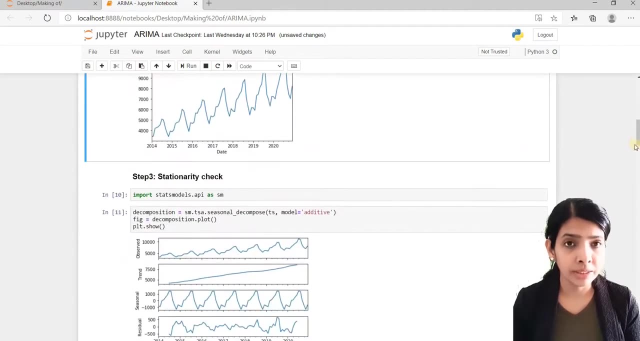 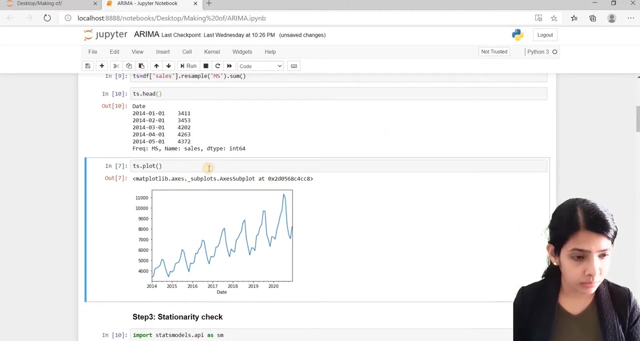 So we can see the month beginning of all the months And it will show the total sales value. Though it is showing the month beginning, it's not that day's sales. It has total sales for that month. Now we would plot the time series. 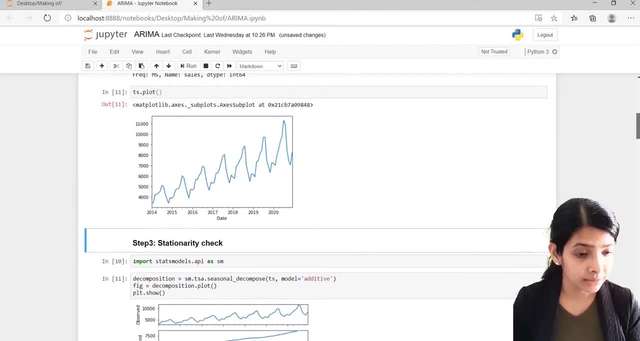 We can see that our time series, the sales, is increasing And we can also see that this regular periodic movements, that it has seasonality in it. Up to this, this was the pre-processing that is required for modeling. From now onwards, we are moving into 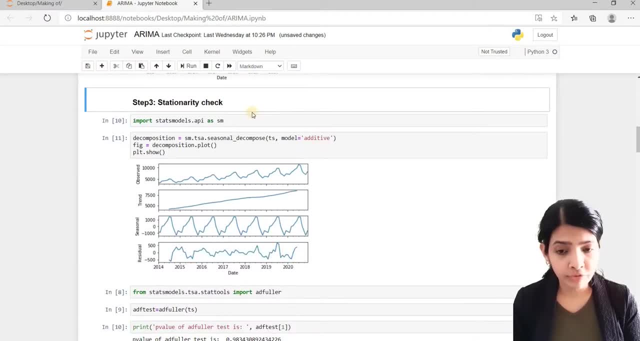 Modeling of a time series. So step four is check for stationality. Now what is stationality? Statistically speaking? a series that has a constant mean variance and autocorrelation over time. That means the series is stationary. 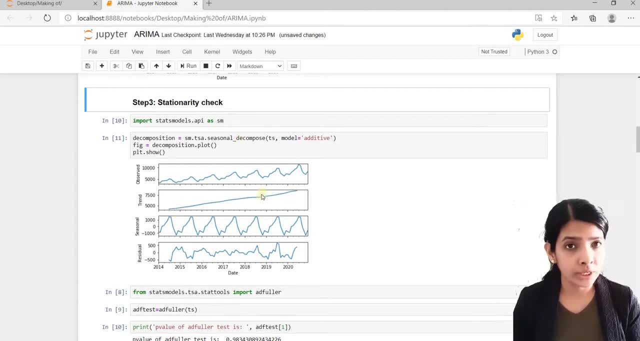 Logically speaking, if a series has no trend or no seasonality, that means the series is stationary. But this series it has trend as well as seasonality, So this series Is not stationary. This is a non-stationary series. 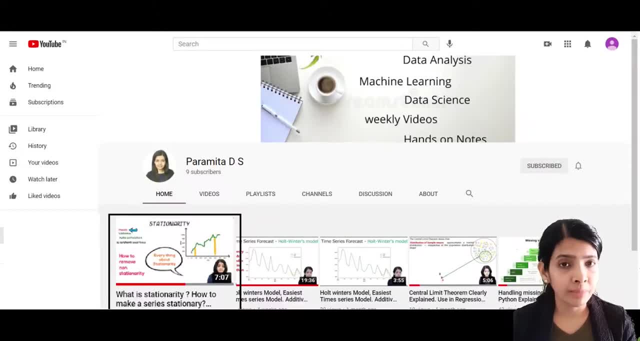 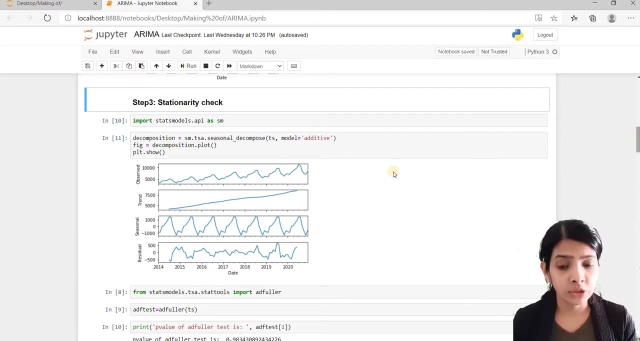 Now, if you want to know everything about stationality, please check my video on what is stationality. It will give you everything that you need to know about stationery in details. Now we have to pay attention to this. The primary assumptions of Arima, or seasonal Arima, forecasting is that we have to make the series stationary. 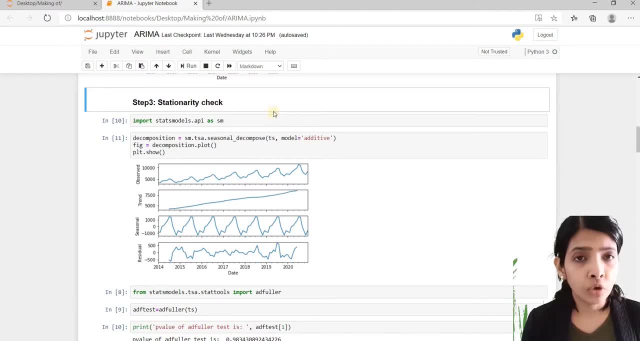 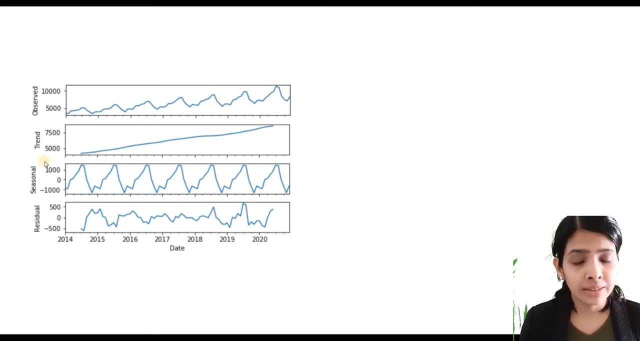 Then only we can do the forecasting. So for forecasting we have to make a series stationary by removing trend and seasonality. Now one might think that trend and seasonality are the factors that we actually want to predict in the future. So if we are removing it, then what are we left with? 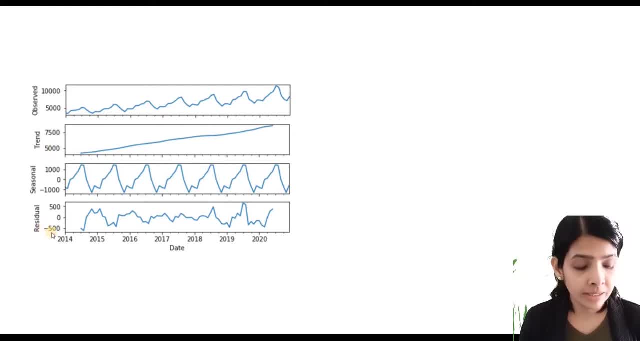 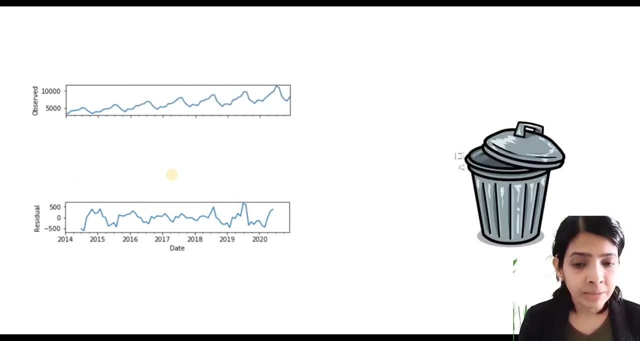 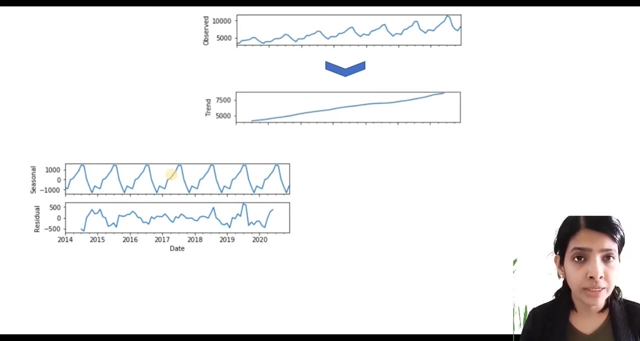 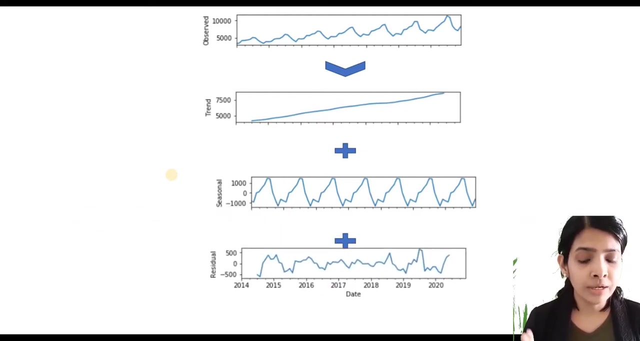 Just a random part. So by removing it doesn't mean that we are removing the trend and throwing it away, or removing the seasonality and throwing it away. Rather, it means that we are taking The original series and we are separating the trend component. by removing it says we are separating the trend component and we are separating the seasonal component till we are left with the random errors. 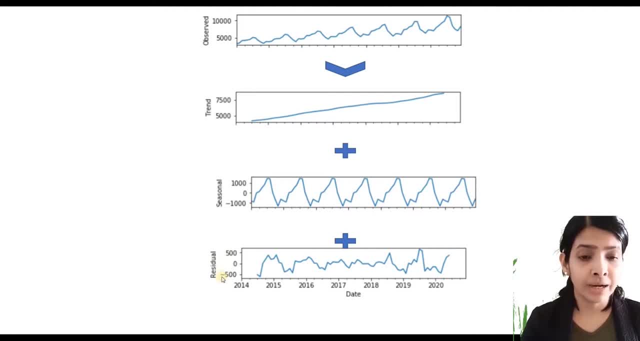 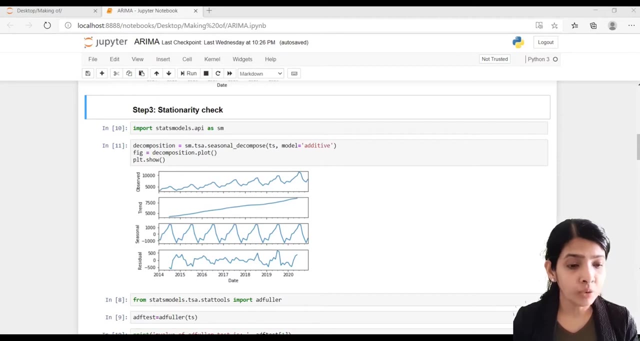 So we have predictive capabilities separated and when we separate these so we can use this trend components and the seasonal components, that is separated, We can use these components to predict the future. So before going forward, let's see That how we can visually separate the trend and seasonality. 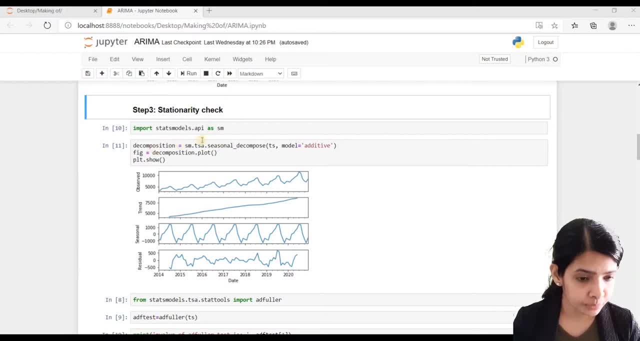 We can do that by using, by importing statmodelsAPI as SM and decomposition is equals to SMTSASEASONALDECOMPOSE. We would pass our time series and give model equal to additive And if we plot this decomposition, then we can see that it has decomposed the observed series into trend and seasonality and the residual part. 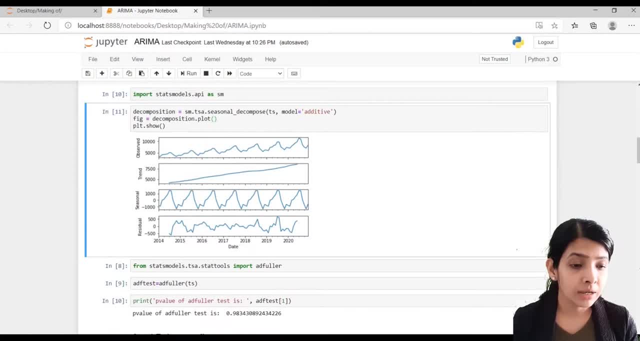 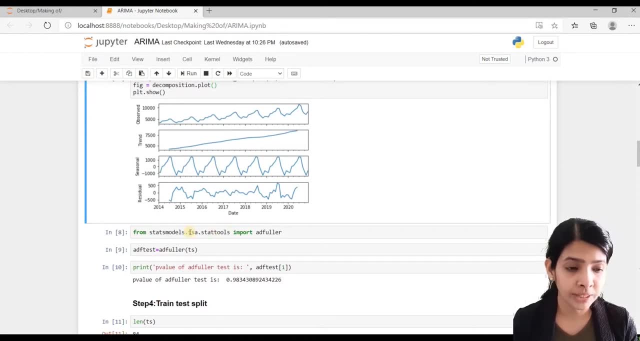 After doing a visual check, we had said that because our time series has trend and seasonality, it is non stationary. But there is a statistical test that we can do that is called AD Fuller test. that says that if a series is stationary or not, for that we have to import AD Fuller from 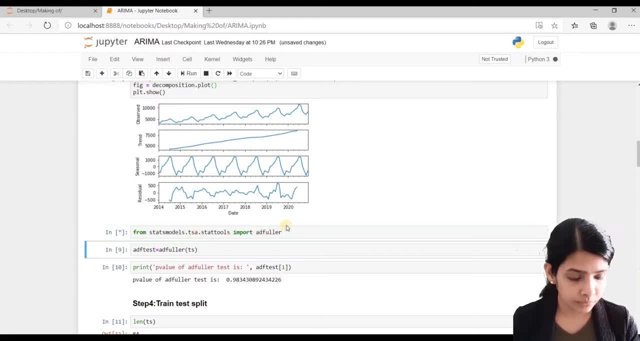 statmodelsstat tools. If we pass our time series in AD Fuller and if we print the result of ADF test, we get a p-value, and a p-value that is greater than 0.05 refers to the fact that the series is not stationary. 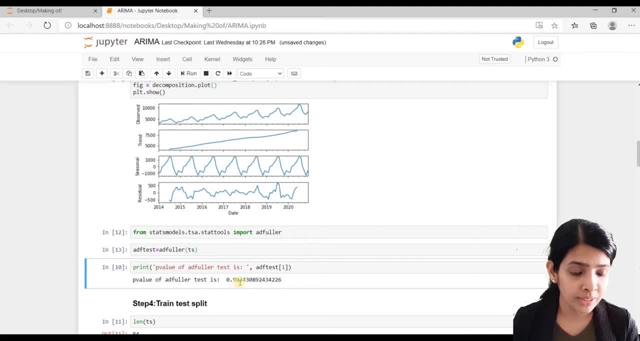 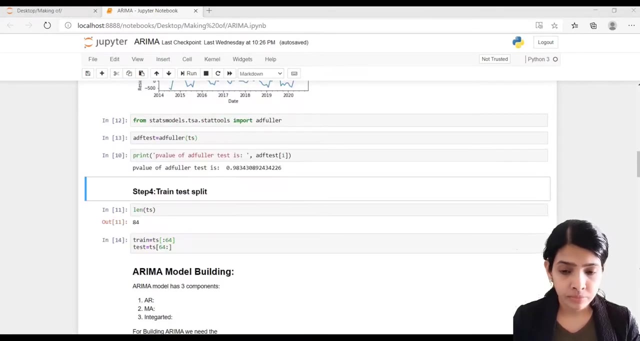 So here we can see it's much greater than 0.05.. That means statistically also we can say that time series TS is not stationary. Now what to do with that and why should we do that? I'll come to that after we do a train test. split of the data. 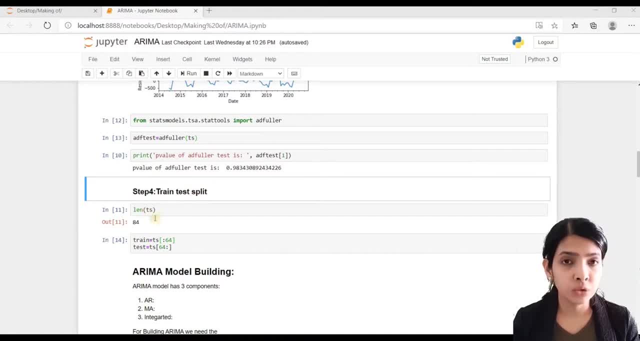 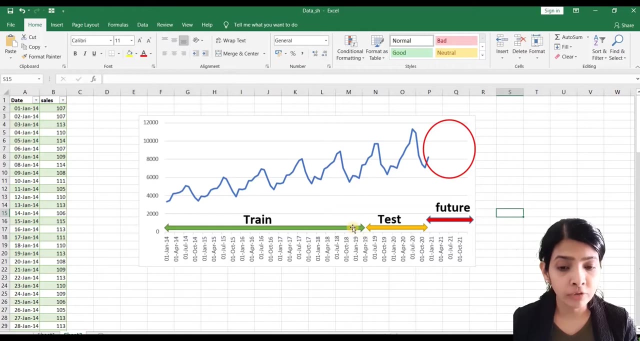 In train test split we divide the full time series into a train component and a test component. We would build our model on the train data. that is January 14 to December 13.. Using that model, we would predict the sales of the test portion of data. 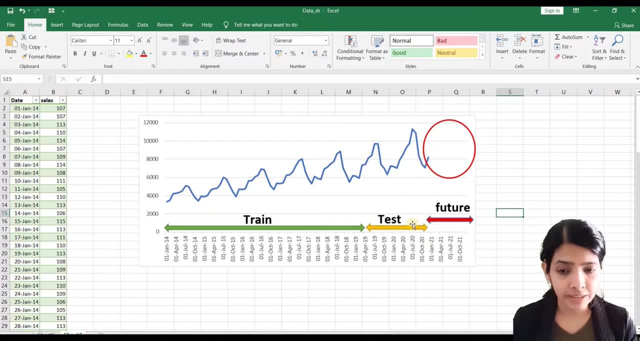 So we can say that the sales of the test portion of data is going to be from April to December 2020.. So for the test set we have the actual sales and predicted sales. Now we can calculate that how far our model's prediction is from the actual data. 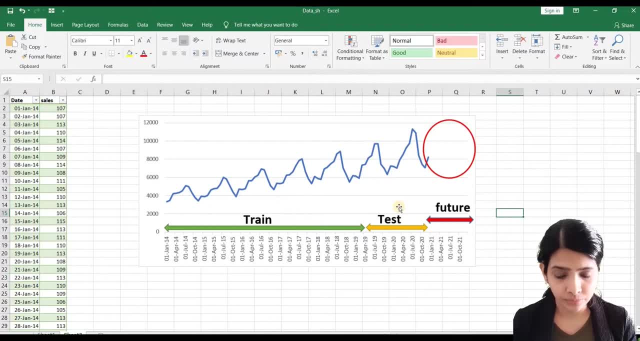 And based on that we can perform a model evaluation and we can say how good our model is. Now. the red part is January 2021 to October 2021. That is the unseen future. That is our primary goal to predict And after we have reached our final model, we would build a model based on the entire data set. 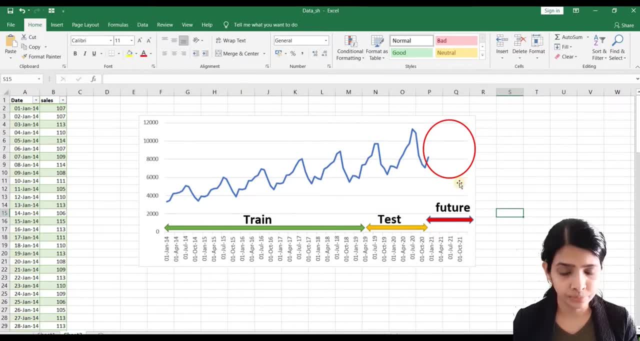 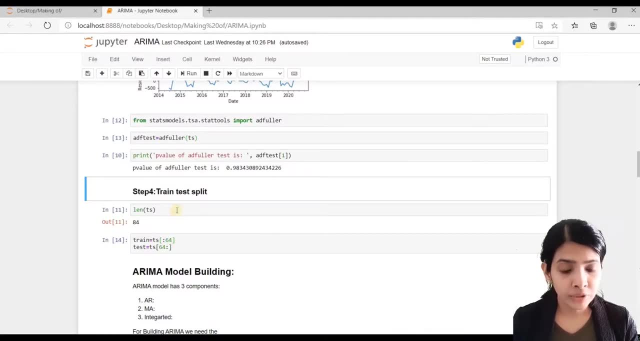 And then we would use that model to predict the unseen future. So for that I would do a train test split by using simple Python subsetting. We write TS and within square bracket say colon 64. That means it takes 0th month, that is January 14, to 63rd month. 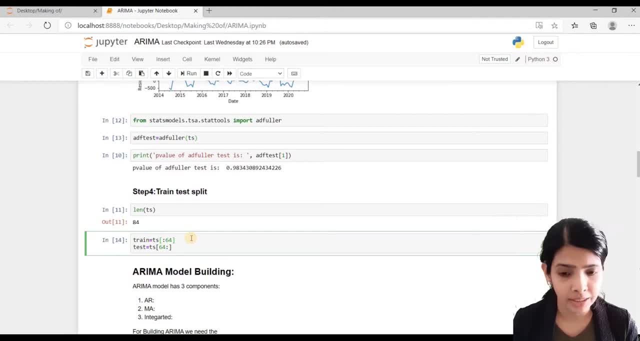 That is, April 2020- 2019 in the train data set. Similarly, we would subset out 64th month to the last month, that is, December 2020, as our test data. Now we would build ARIMA model on the train data. 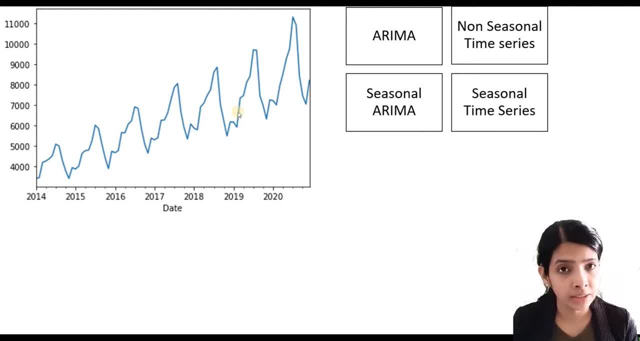 Now let's look at the time series. once again, I've seen that it has trend and seasonality. If our time series has seasonality, then we should apply seasonal evaluation ARIMA, as in only ARIMA, we cannot capture the seasonal seasonality. 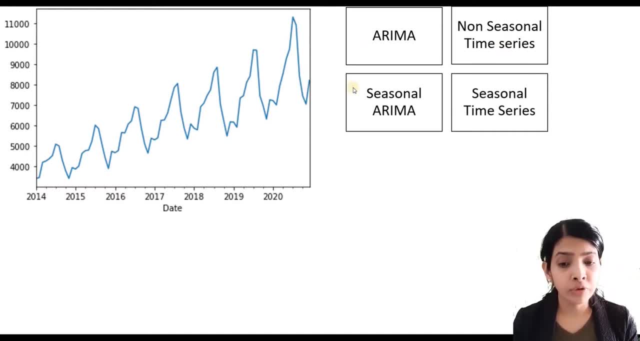 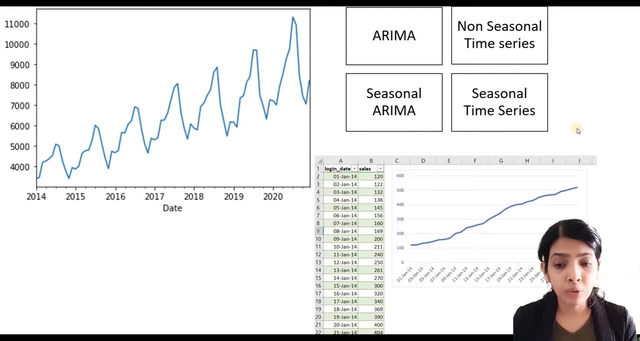 But here I am still implementing ARIMA on this model so that when I implement, when I apply seasonal ARIMA to it, you can be able to see the difference clearly. But I'm also giving you one more data set for practice of ARIMA model. 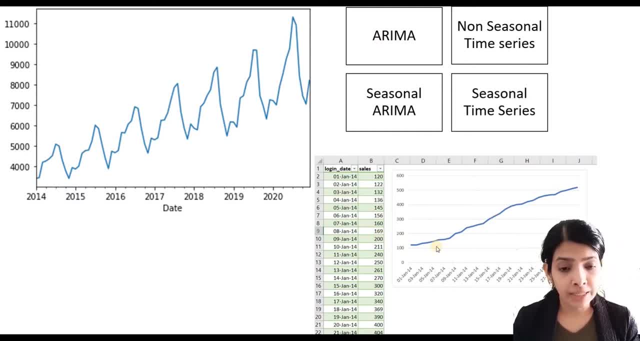 The link is given below in the description box And for that time series you will implement ARIMA because it has no seasonality, It has only trend. This is for a practice data set that I'm giving you Now. ARIMA has three components. 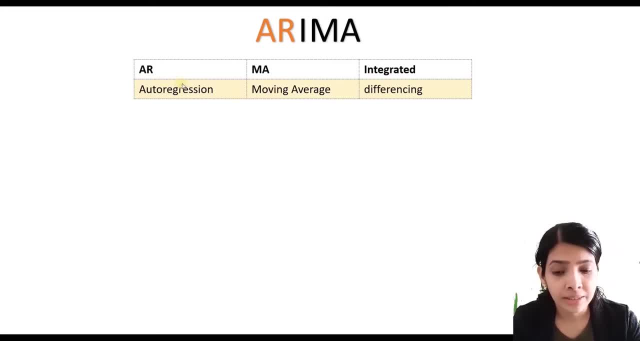 AR, that stands for auto regression and it means that regression with its past value within the same series. And if a model is an AR model, that means that the sale of December is correlated with the sales of November and October, etc. Now, how many past months should we consider? 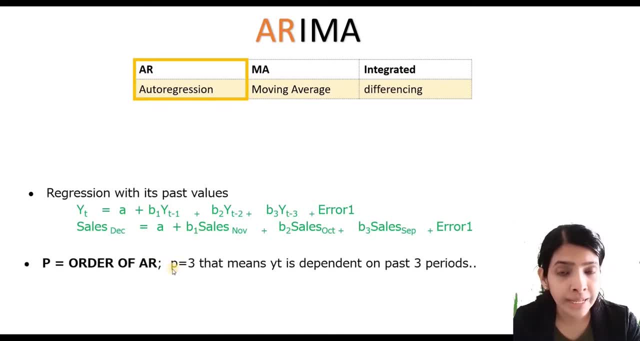 That is called the order of AR model and denoted as P. So for a order 3 AR model, that is AR3 model. the mean sales of December is dependent on last three months. Similarly, the sales of November is dependent on October, September and August. 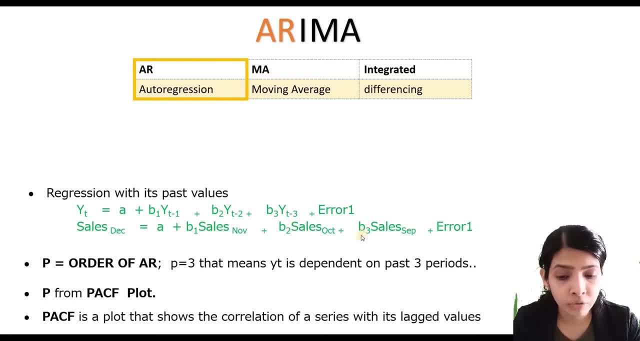 So in AR model, the model finds the correlation with its past previous lag values and use those lag values to predict the future. But technically, how are we going to find the order of the AR model? There are three methods of doing it. 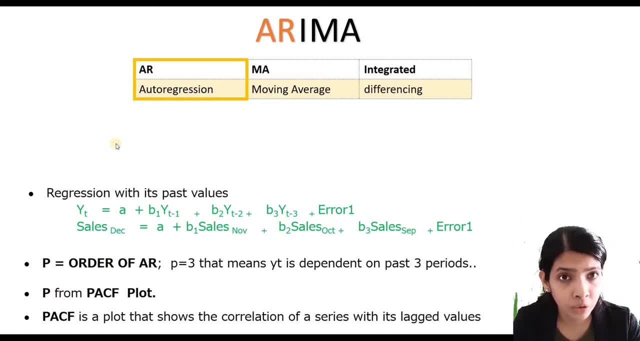 And I will talk about all the three methods while we are in the coding part. But the classical method is by using a plot called PACF plot. I will discuss about it during the coding, But we will not use PACF plots. We would use a more result driven way of identifying the orders. 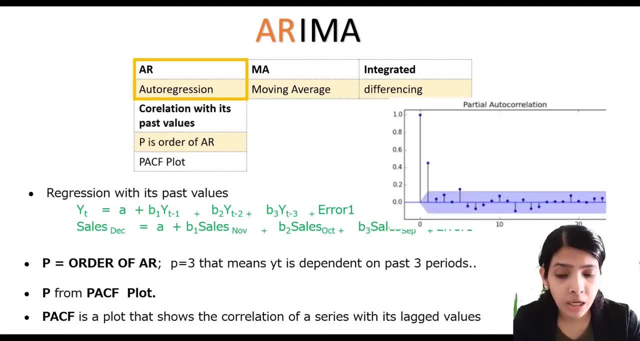 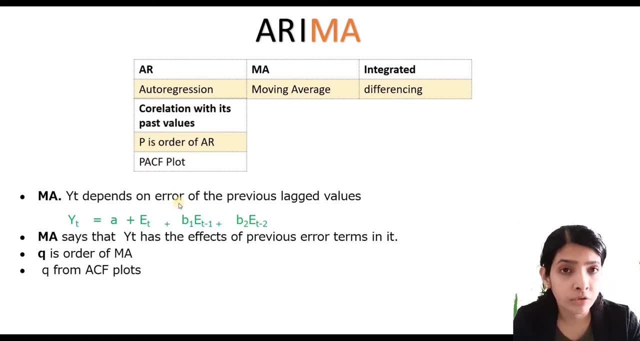 So the second component is the MA component And in MA model says that the present values of a time series model are dependent not only on its past values but also on the error of the past values, Like when we did an AR model that was an auto regression. 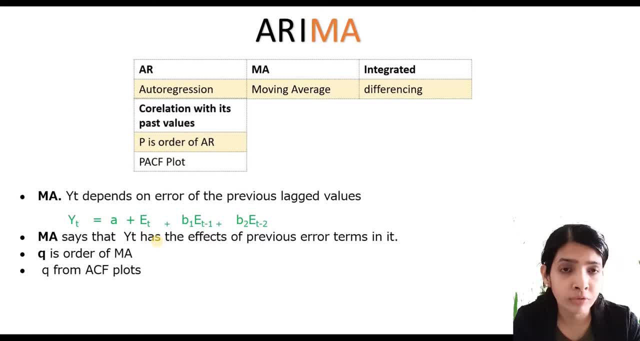 So whenever we do a regression, we have an actual value and we have a predicted value, And the difference is the error. So the error that is coming out of auto regression model. MA says that the current value is also dependent on the error terms. 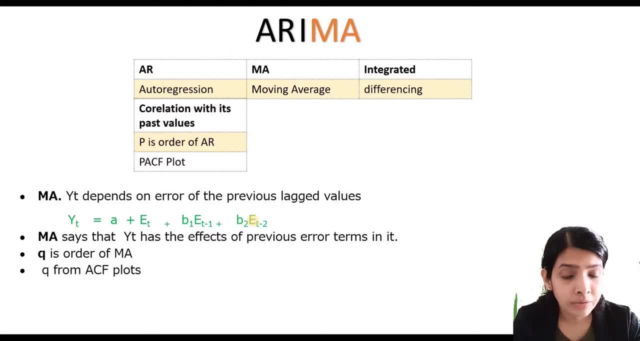 So we can say that current value of y is dependent on the error terms of previous lag values. But how many previous lag values error can be used to predict the yt? That is the order of MA and that is denoted by q. We can find q by using a plot called ACF plot. 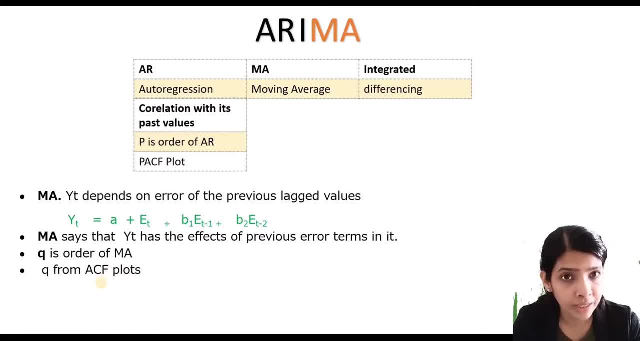 And that this is the classical way. But, as I told you in case of AR also, there are other three methods of finding it And I will show you the best method, as per me, that gives better results than ACF plots. The third component is I. 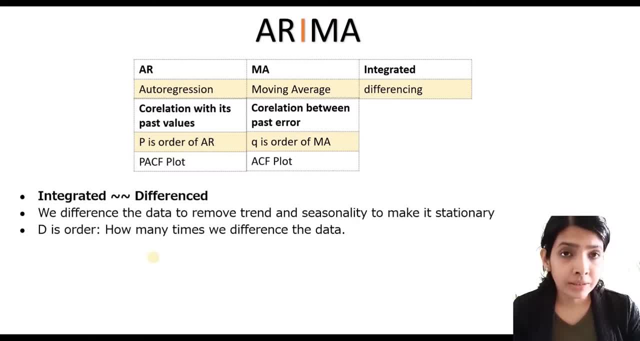 I stands for integrated. Now, integrated, this term comes from differentiation. We know that we have a concept called differentiation and integration And differentiation. if we differentiate something, it means that we subtract the sales of December by sales of November. We are just subtracting the values of one time with the previous time. 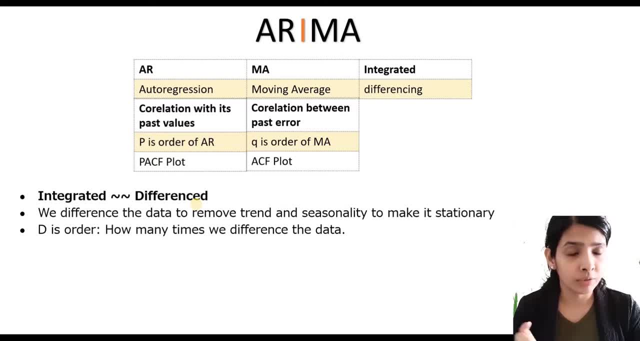 So we are differentiating the values and by doing a difference of previous values we can eliminate the effects of trend and also seasonality. So we difference the value to remove the trend And we as we know that to achieve stationality we have to remove trend. 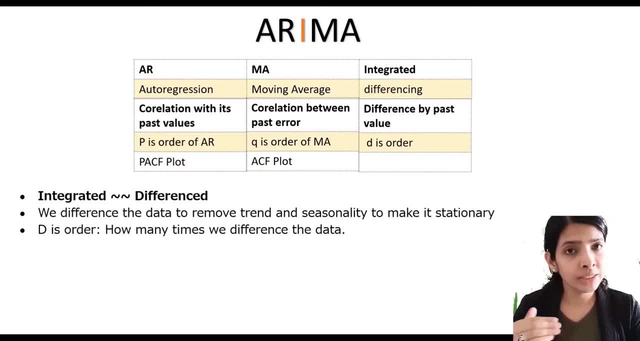 So this is what is called differentiation. But when we are differencing the data, the original series is getting changed to a different series. Integration stands that when we difference the data, we integrate it back to go back to the original series. So basically I, integrated means difference. 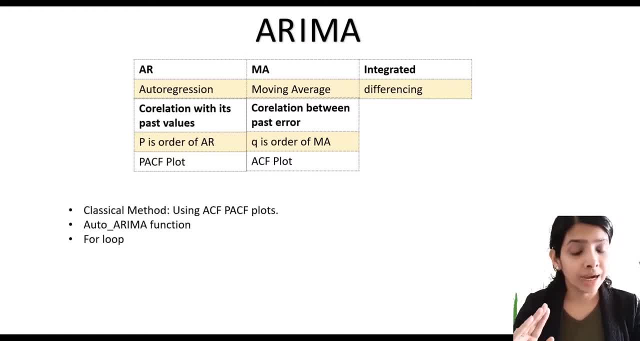 In the other way round. So basically, integrate equals to. if I say I integrate by one, that is, I subtract one value with just its previous value, That means we actually have differentiated it. And to get back to the original series, I'm integrating it to one. 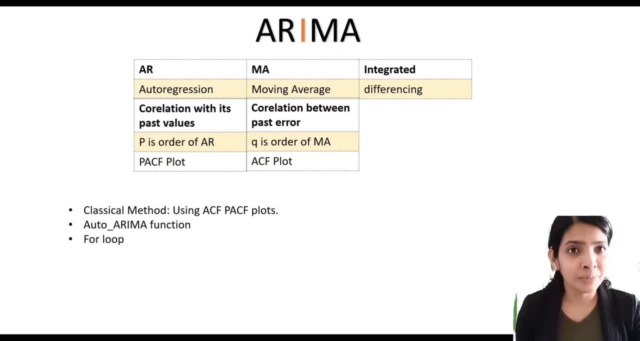 So technically it should be called difference, not integrated. But as we are integrating it back to get the original series, that's why it is called I, That stands for integrated. But how many times We need to difference a data to make it stable? 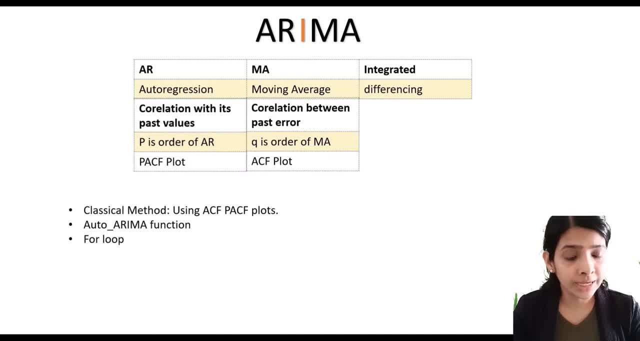 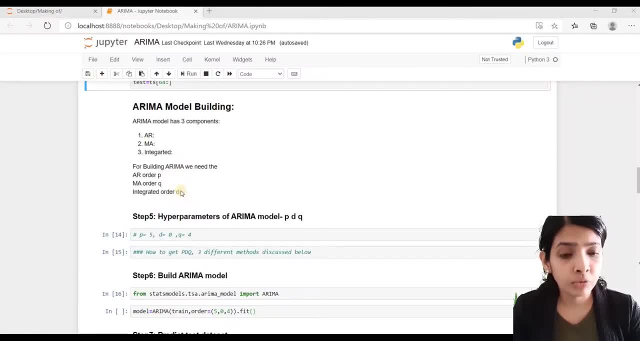 That is also another hyper parameter that is called D And we also have to find out, And there are graphical ways of doing it And there are other technical ways of doing it. We would see both of it. So now we know that to build model for AR part. we need a P order for MA part, We need a Q order and I we need to know how many times we have to differentiate the data to make it stationary. So there are three parameters: hyper parameter, that goes for ARIMA model, that is, PD and Q. 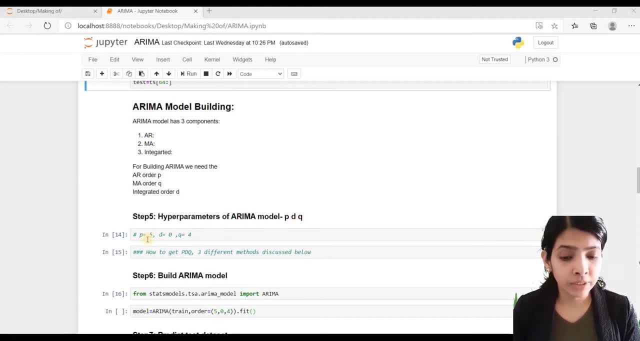 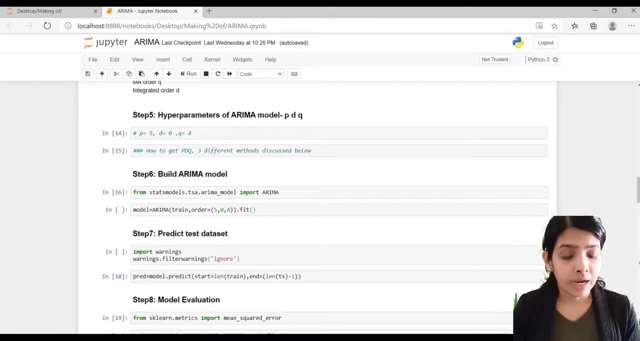 Now you can see here that I have written: P equals to 5, D is 0 and Q equals to 4.. Now how did I get these three? I will talk about it in details after building the model in a separate segment. 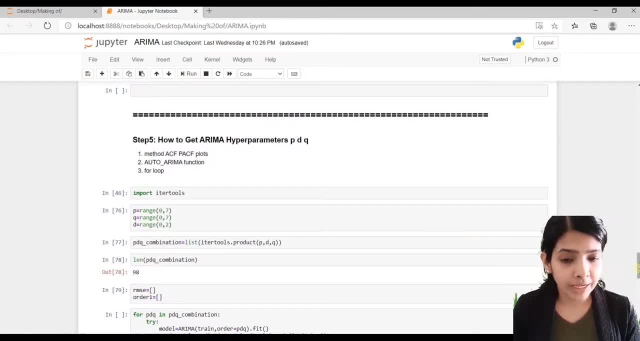 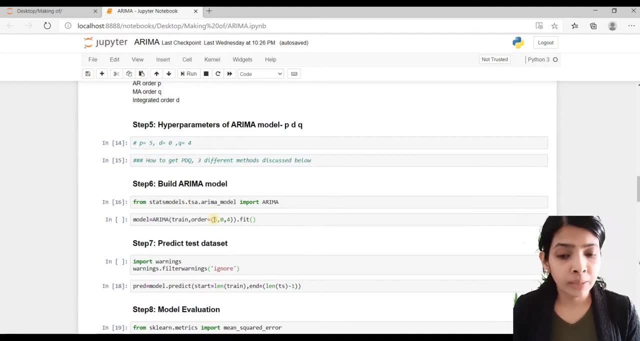 But for now, let's assume that I have Got these values by some magical power. I know this, Okay. So now, by magical power, we know that P equals to 5, Q equals to 4 and D equals to 0.. 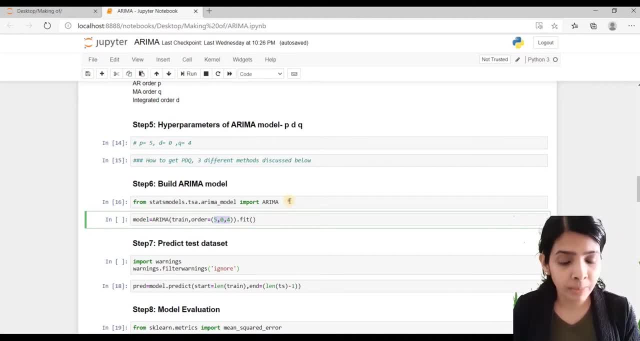 That gives our ARIMA model. Now we would build our ARIMA model on these hyper parameters, And for building ARIMA model we have to import ARIMA from statmodeltsa. ARIMA model We would write: model equals to ARIMA. 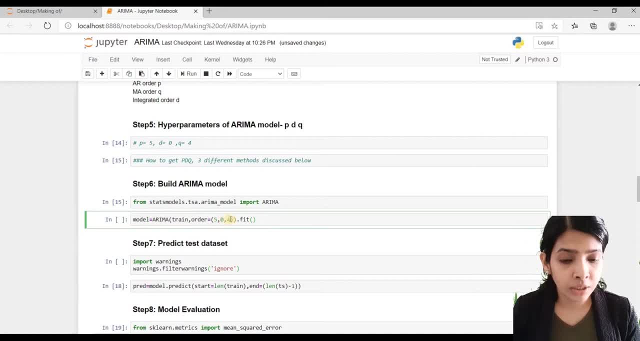 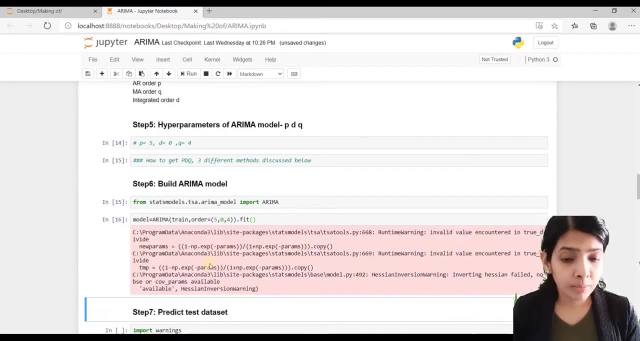 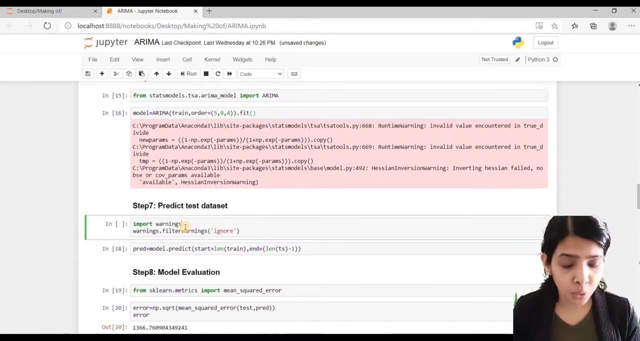 We pass the train data set and, within order, we give the orders of P, D and Q and we fit the model. You can see that there are some warnings that are coming and we can remove these warnings by using Import warning warnings. filter warnings ignored. 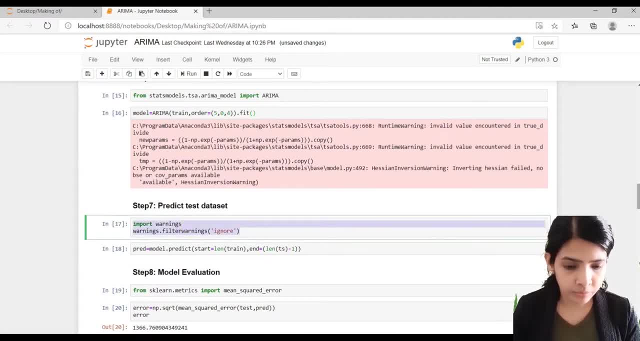 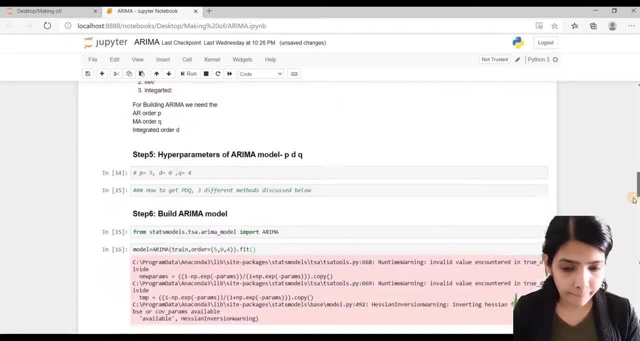 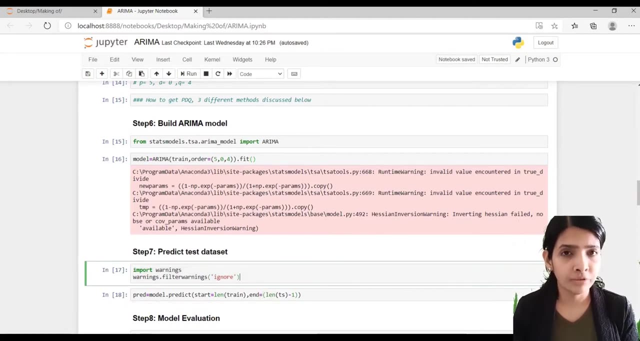 If I run this, I should have pasted it above, And then, if we run it, the warnings won't be Displayed. Now we have our model. We have to predict the values for test data set so that we can do a model evaluation. 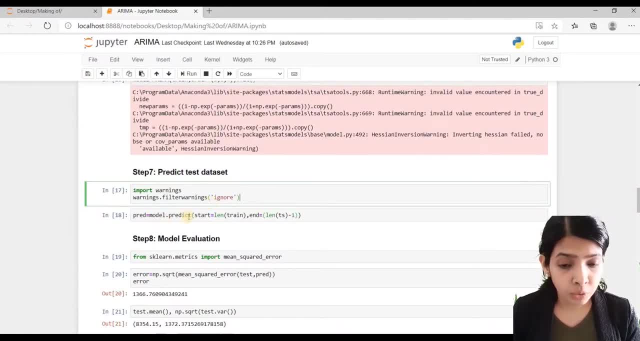 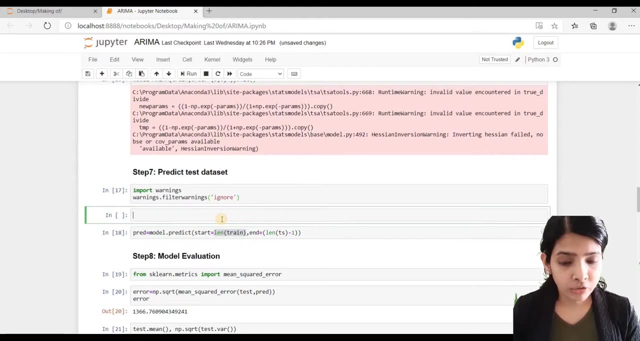 And for that we have to, we use model dot credit function and we have to start, give a start and end parameters That would say that from which period to which period? what is the length of the predicted data set? So length of train is 64.. 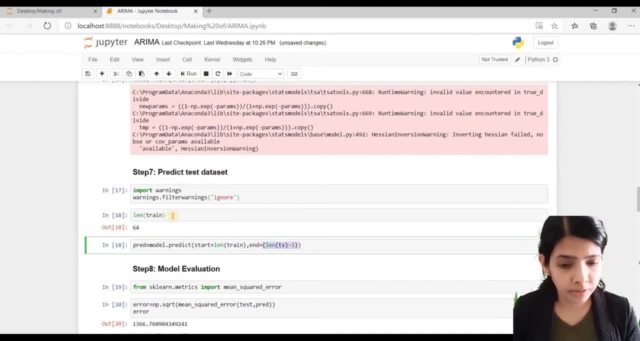 That means it would start predicting from 64th month to the length of DF, Subtracting it by one. Otherwise it would, you know, exceed the length of the test data set. We are just here trying to build a data set that is of same dimension as the test data set. 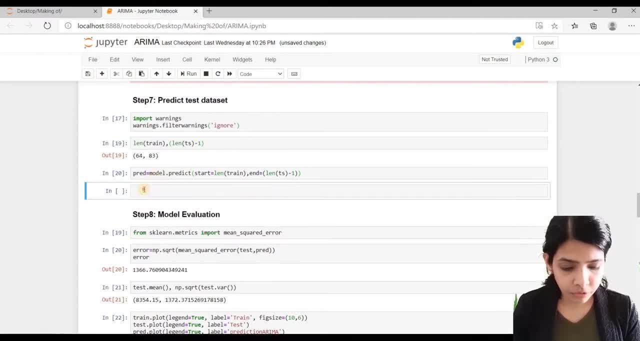 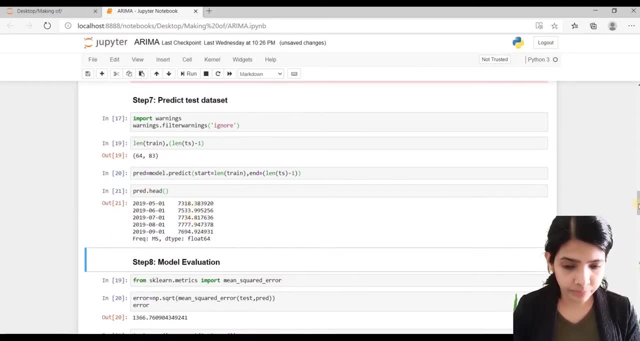 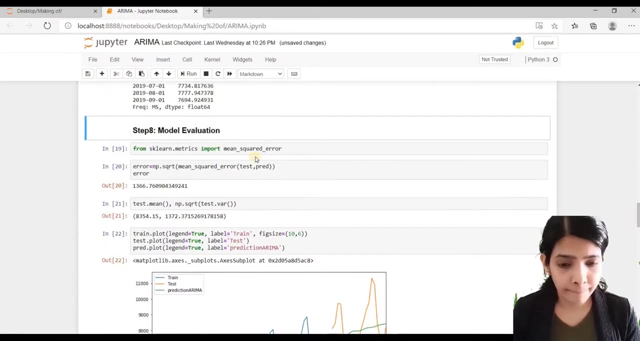 We have our predict. If we see pred dot head, We can see that the month wise prediction is here. Now, based on that predicted value, We would evaluate the model, that, how good our model is. So for that we need mean squared error imported from a scale under matrices. 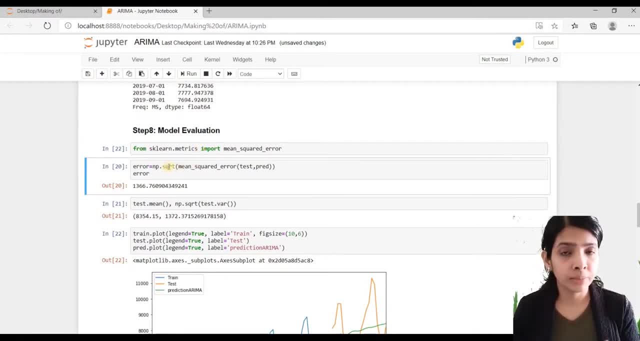 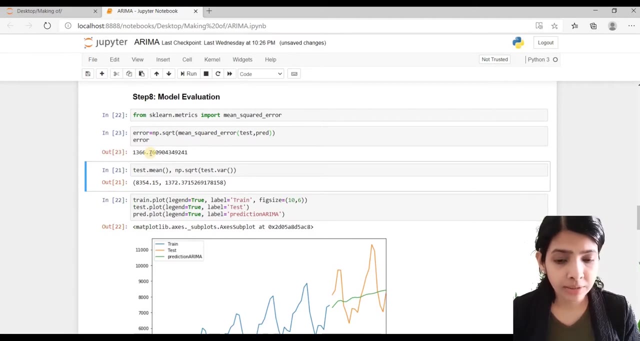 So we would do a root mean squared error will pass the predicted and true values and find that how far our predicted values is from the true values, And I would save that in error. So the error is one three double six. Now what does this one three double six means? 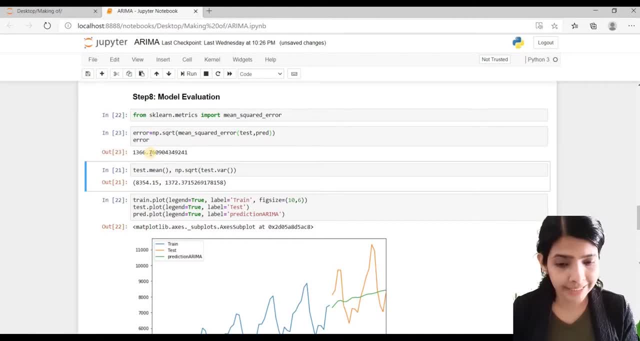 Is this a good model or not? One way of finding that out is if we find the mean value of the test data set, and by here I am writing test dot VAD and taken a square root. That means this is the standard deviation of the test data set. 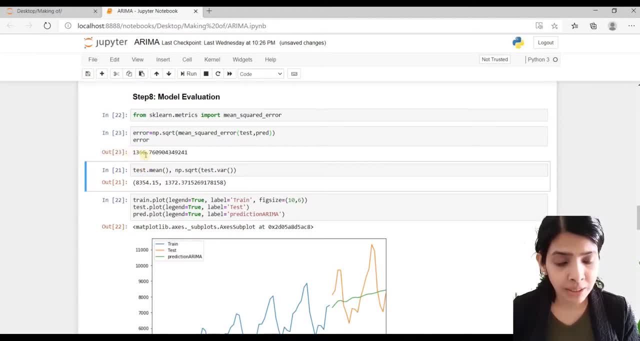 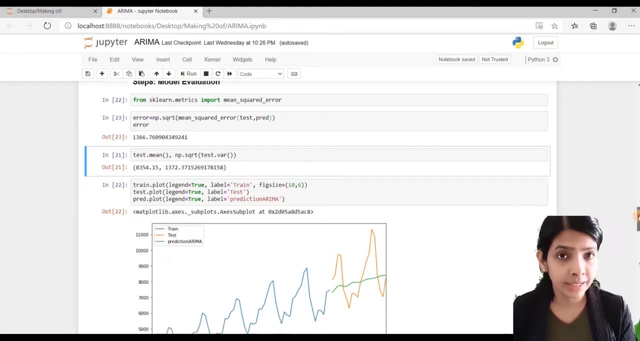 So we can see that our predictions is within one standard deviations away. This is not a very good model, but it's not doing very good because we have not captured the seasonality part of it. So it's a okay model, not a very good one. 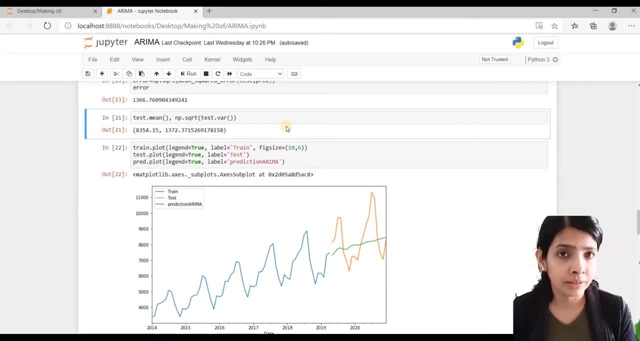 We could have made a better model that we would do after edema. We will make the seasonal edema and that would give much less error. And here I am plotting the train part. This is the train data. The test part is the orange part is the actual test data. 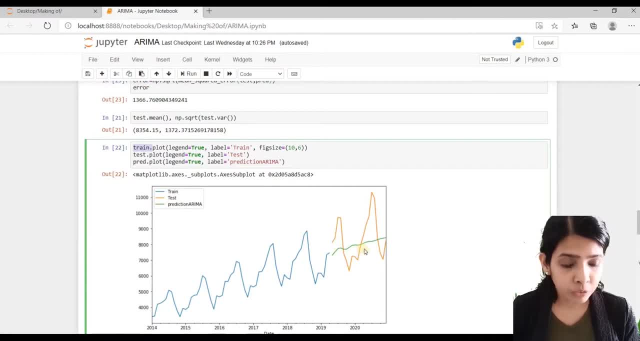 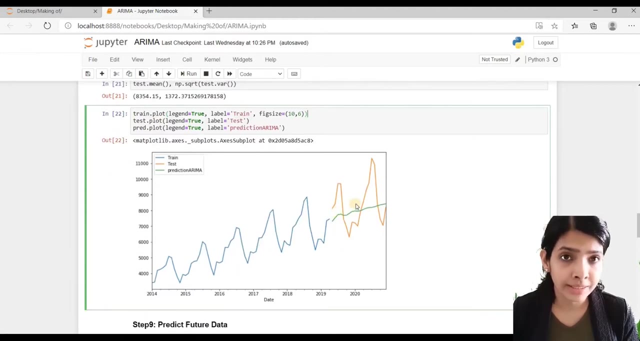 And the predicted part is the green line. So we can see that, as edema cannot capture the seasonality, It is just capturing the trend increase of the data. So edema forecasting will always give a forecast like this. It will never capture the seasonality, like in case of seasonal edema. 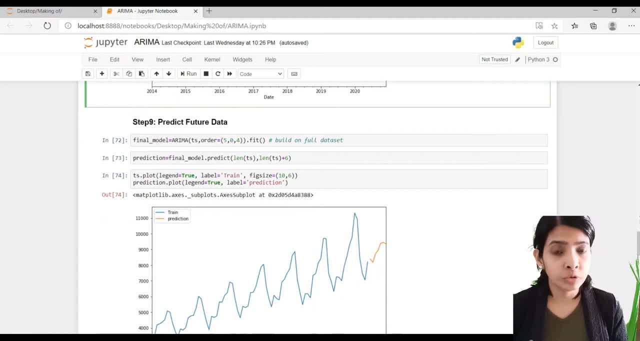 Step nine we would predict the unseen future data, And for that I am not using the model that I have built before. This model I am not using because here I have used the train data When I have finally got my actual final model. 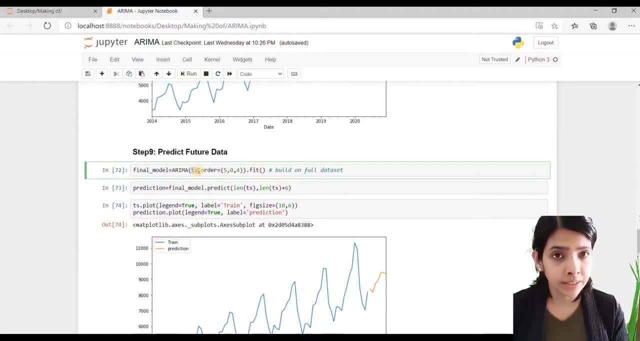 I would use the entire data set, that is the TS, to make my final model And I would give the same hyper parameters that I have selected and I will build the model. Then I would use final model dot predict, to predict the future. I will start with the end of the data set, that is, from December 2020.. 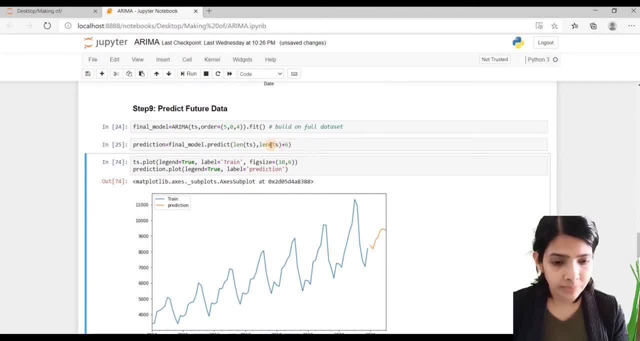 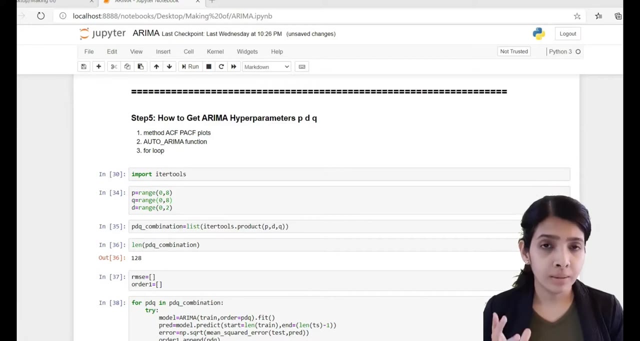 To next six months. That's why I have given plus six, And that would be saved in prediction. Now I am plotting the entire time series and also the prediction for the unseen future, And this is how it looks like, Now that we know how to build a model. 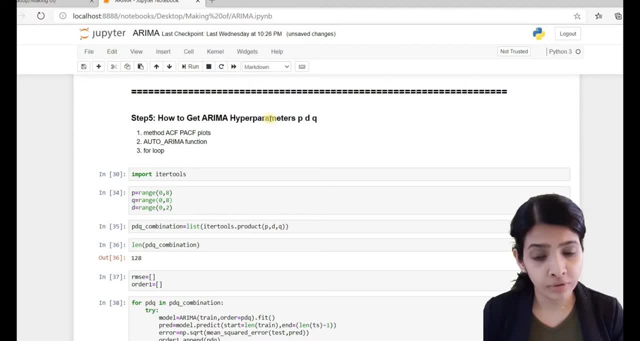 How to get the prediction and how to evaluate the model. One thing that we have left was how do we get the hyper parameters PD and Q? Now there are three methods of getting it. One, by using ASafe and PSAfe. That is the classical and most talked about method. 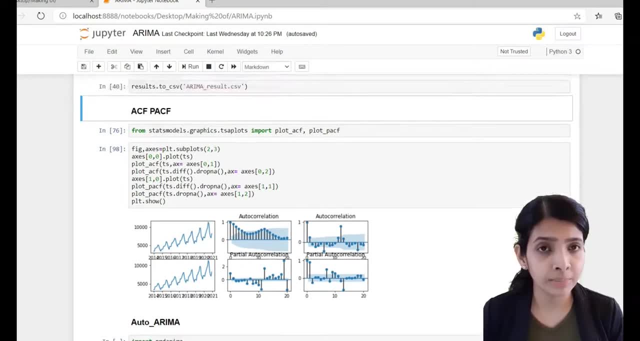 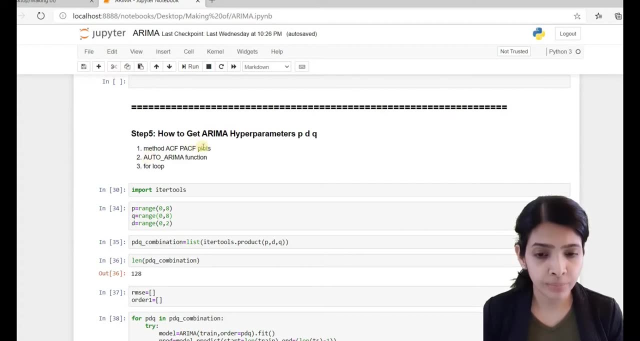 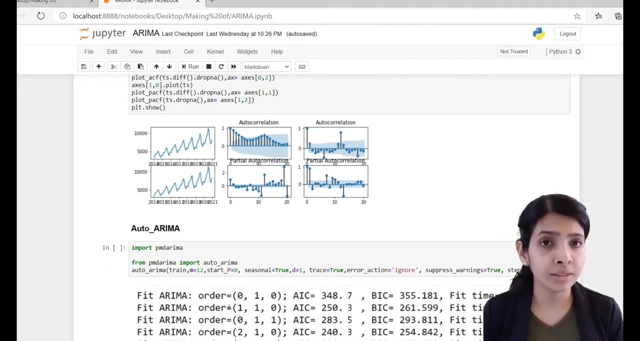 But ASafe, PSAfe plots are very complicated plots to understand And one should not solely depend on ASafe and PSAfe plots. In this lecture I have shown you how we can get the ASafe and PSAfe plot, But I am not telling you what are the different combinations and how we can come to a conclusion. 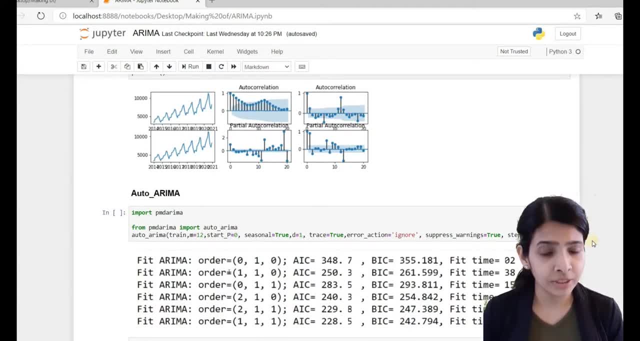 Because it requires a lot of study, And I have a separate video on ASafe- PSAfe plot, So kindly go and check the video if you want more and complete information of these two plots. The method that I am showing here is a custom for loop. 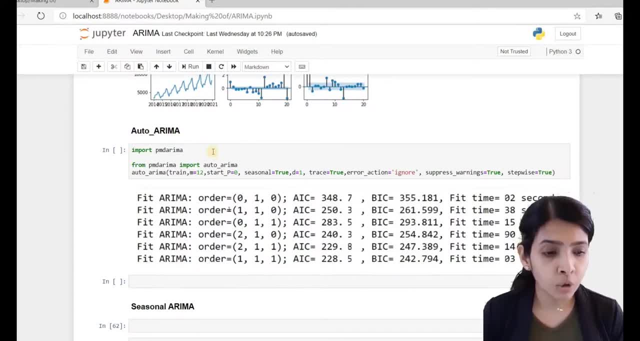 And before that, I will tell you what is auto arima function. Auto arima is a function that is available in PMD arima library And it is an automated function. It fits all the possible combinations of PD and Q And gives the result in terms of AIC and BIC. 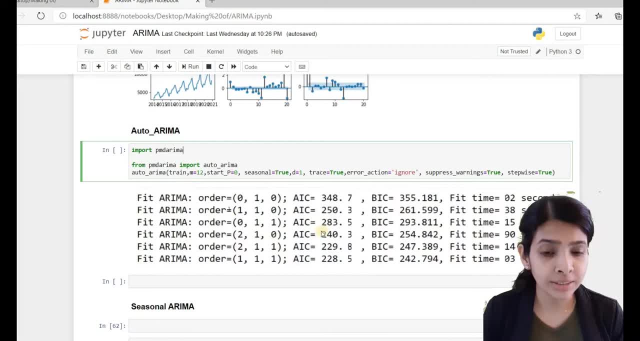 And the best results orders that has the best result is chosen. Now. the disadvantage of this method is that AIC and BIC is not the criteria that we use finally for model evaluation. So a model that has the perfect AIC- BIC might not have the best result in terms of the mean squared error. 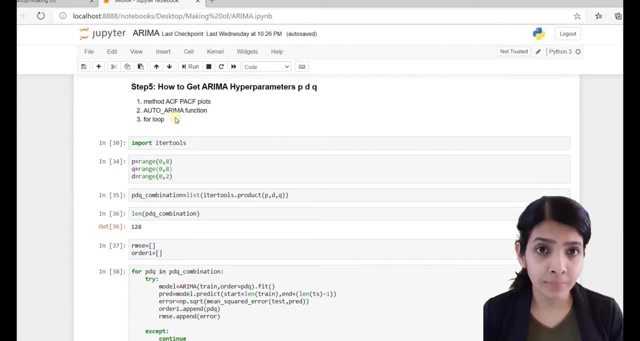 So the method that I have used here and is, in my opinion, the best method out of these three, is using a custom for loop. Now, in this method, what we would do First, we have to import iterative tools And we would give a wide range of PD and Q. 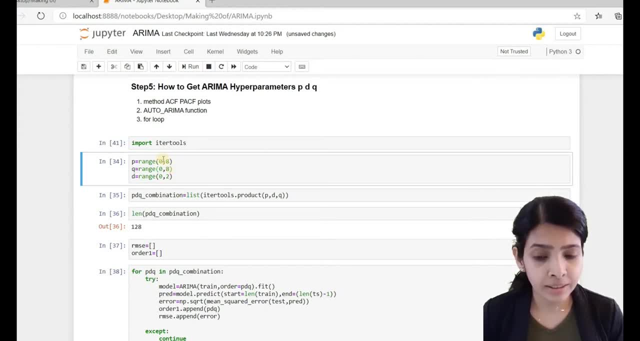 So I am saying that the P and Q can have any values from 0 to 8. And D can be 0,, 1 or 2. Because we don't generally have to differentiate more than two types, So I have taken all the combinations of PD, Q. 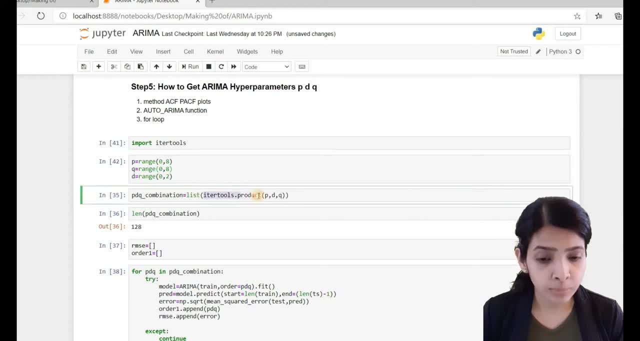 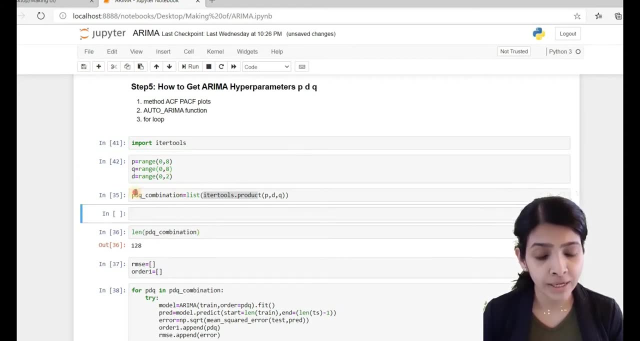 Now run iterative tools dot product. This would give all the Cartesian products all the combinations possible with these PD and Q And we save that as a list in PD Q combinations. So PD Q has total 128 combinations. If you want to see, these are all the possible combinations of PD and Q. 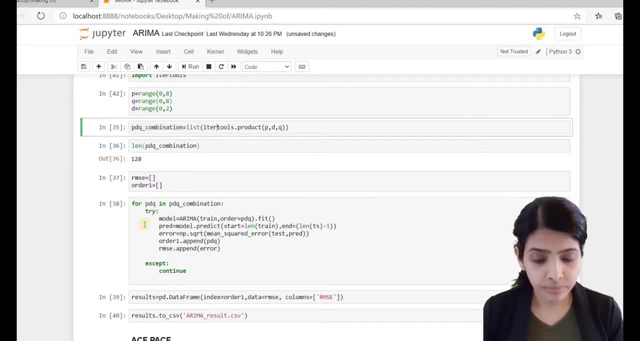 Now I am writing a for loop, But I say that PD Q will run through all the possible combinations Of PD and Q And it will pass that combinations of PD Q in the order of arima. This line of code is what we have used here. 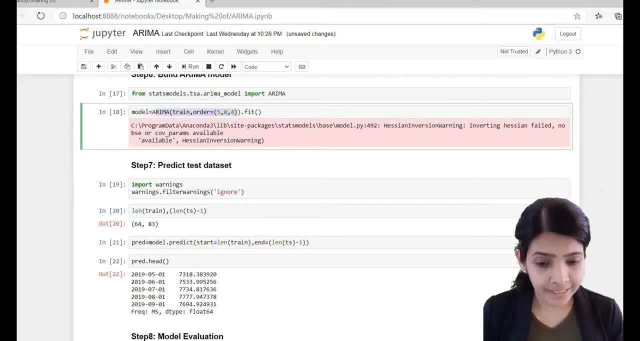 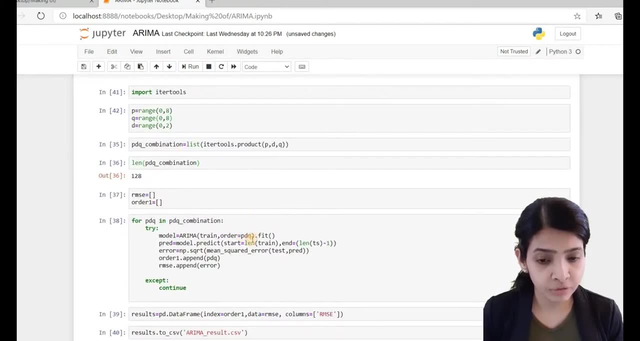 This is the model that we have fit, But here I am not mentioning the PD Q, I am just saying that this can be anything within the combinations of PD Q, So different models on the different combinations of PD Q would be run And saved as model. 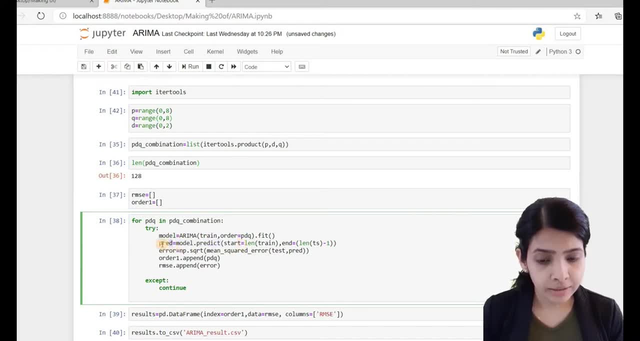 Now this model would be used to predict And that prediction would be saved under pred. Now we would calculate the mean squared error Where we pass these predicted values And pass the test result. that is the test data, that is the actual data And it will calculate the error. 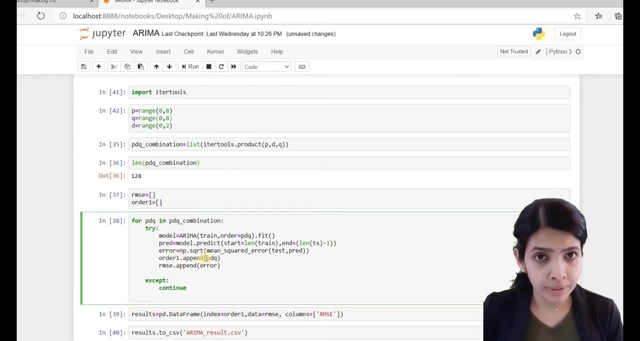 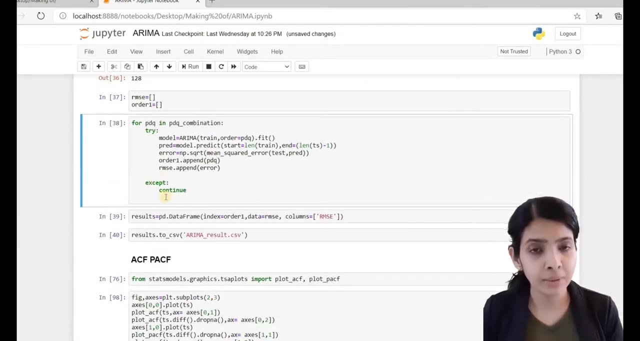 Now we have created RMSC and order, two empty lists. Now orders will be: The PD Q would be saved in order And error would be saved in RMSC. And I have kept all these in try, except method, Because there can be certain combinations that can throw error. 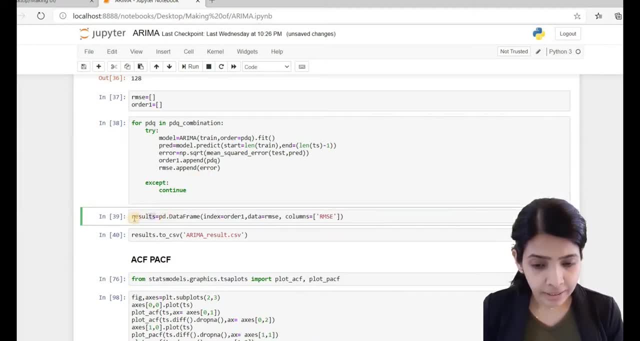 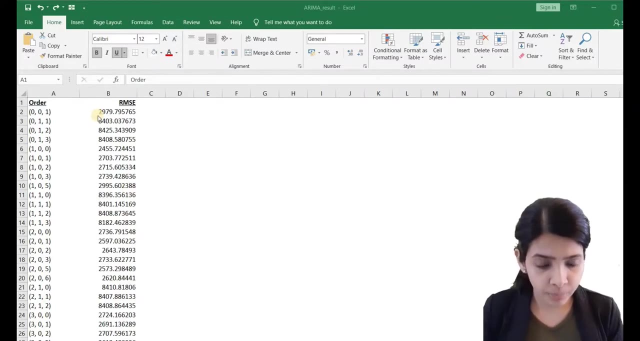 So if I run this line of code And I am saving the results- That is, the RMSC and the order- in a data frame called results, And I am exporting that result in a CSB file. Now let's open the CSB file. 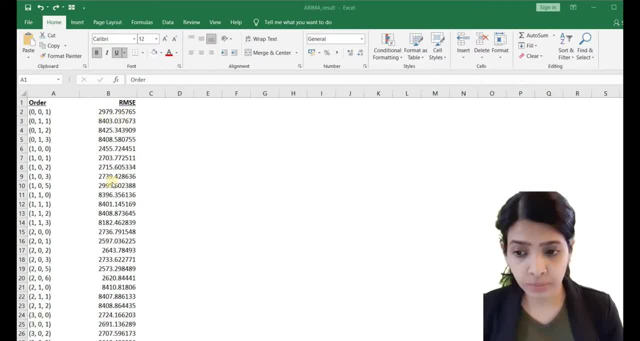 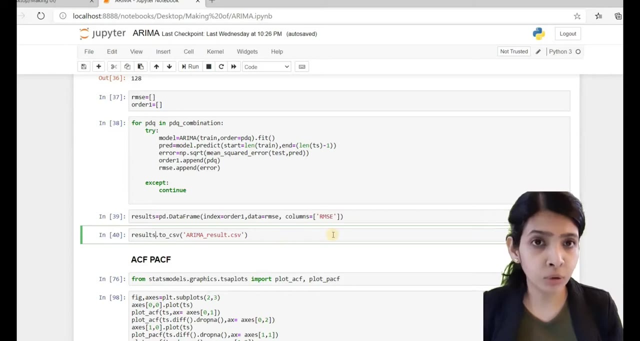 So these are all the PD Q combinations and the respective RMSC. If I sort the data, We can see that this combination gives the least RMSC And this is how I got my PD Q value. And this method has one more advantage. 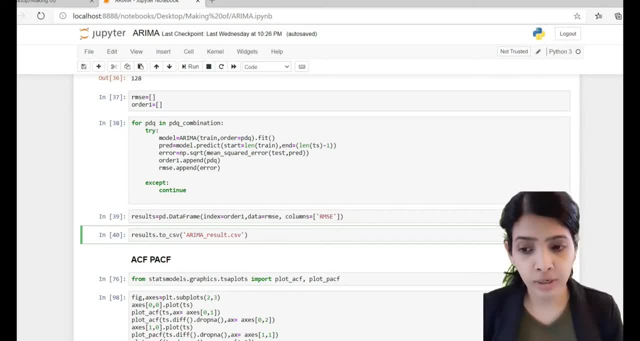 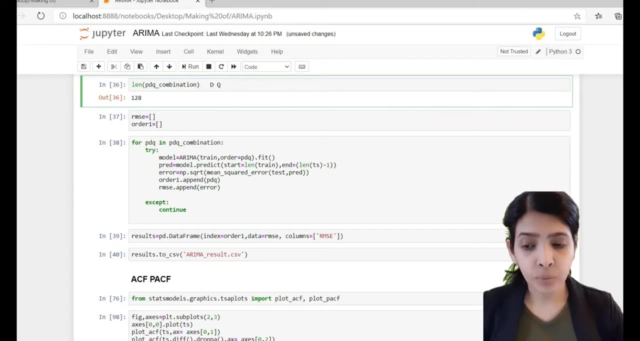 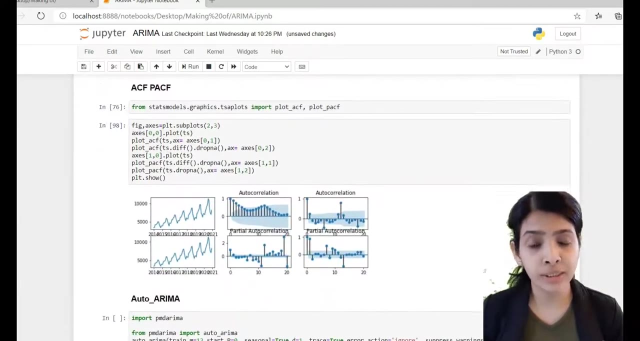 That is in case of seasonal Eulerima, When we would have more hyper parameters like capital PD Q, Then those cases also. We can use this as a tool where we can directly compare the different combinations of PD Q With the root mean square error that they are giving. 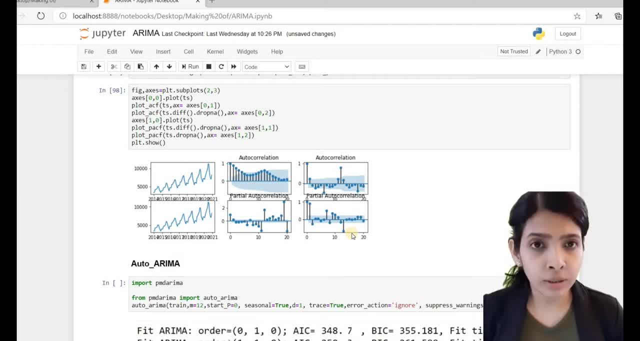 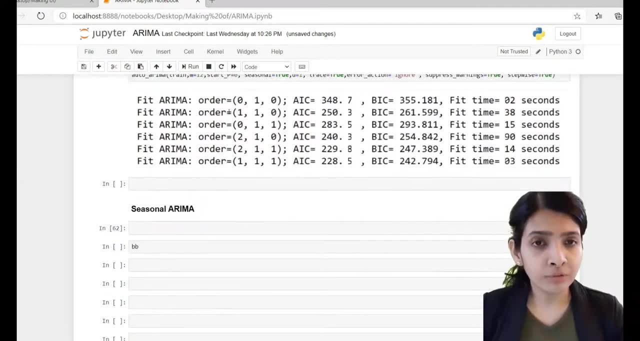 So, and the only thing that I have not covered here is The how to read ACF and PSF plot, Because I think that would be a lot of information bombarded in one lecture, And I have a separate video for that Once you are done. 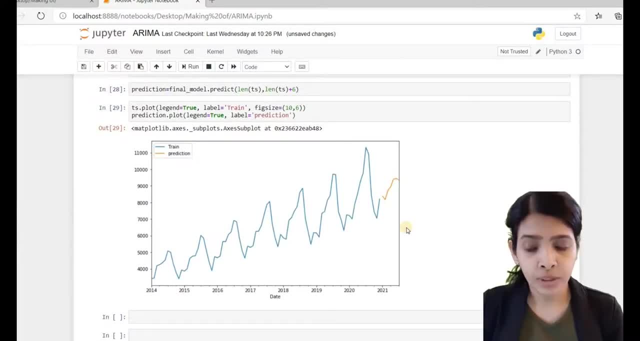 I would suggest you to go and check out that video So you know that, technically, how we can use ACF and PSF plots To identify, or at least cross check with, the results that we have achieved with the for loop. The next step that I would do is on the same data.